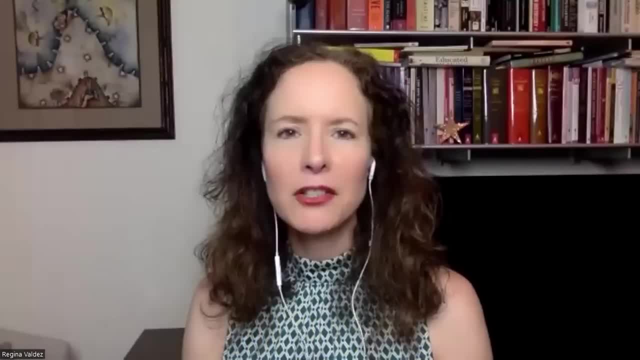 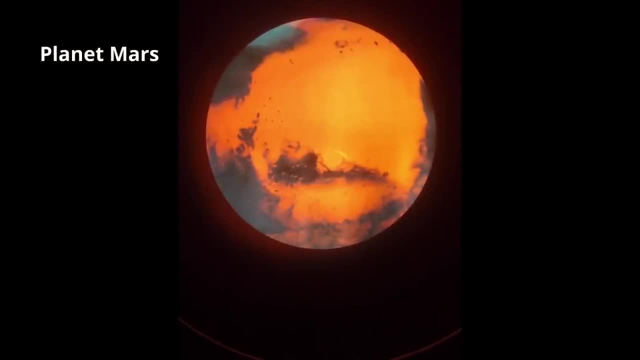 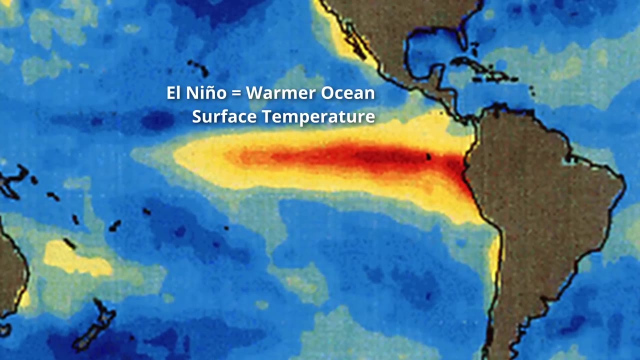 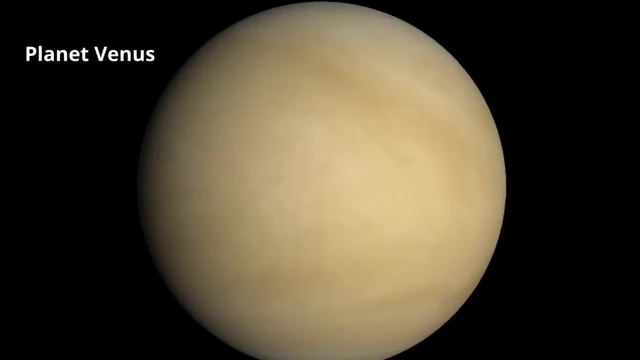 quite a few years ago, trying to help people stay in the relationship. Well, Mars is the red planet. Red denotes warm. So when you think of El Nino, think about where men are from Mars It's red, It's on fire, It means warm. Well, Venus is rather cool by comparison. It's got yellow coloration. 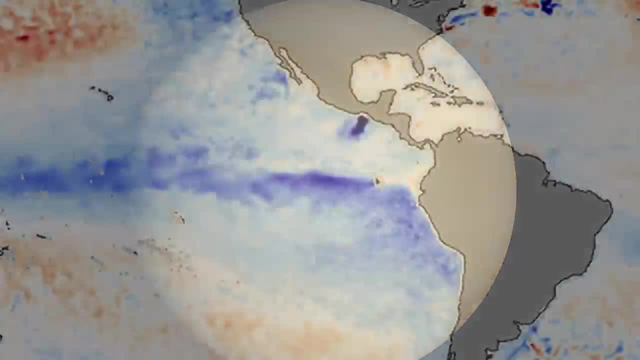 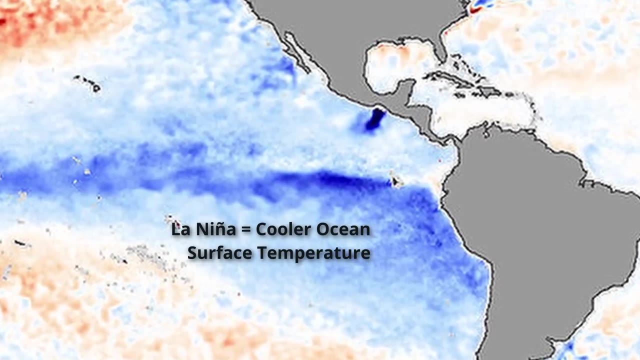 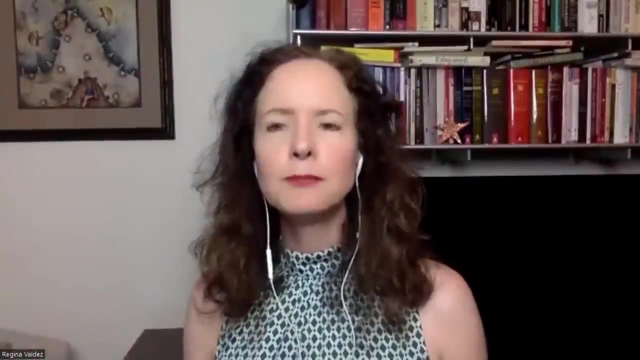 and white coloration. La Nina, the female denotation of the phenomenon, not in the actual sense, is cooler, And La Nina as such is also cooler. These two forces, if you will go back and forth, It's the swinging of the pendulum. 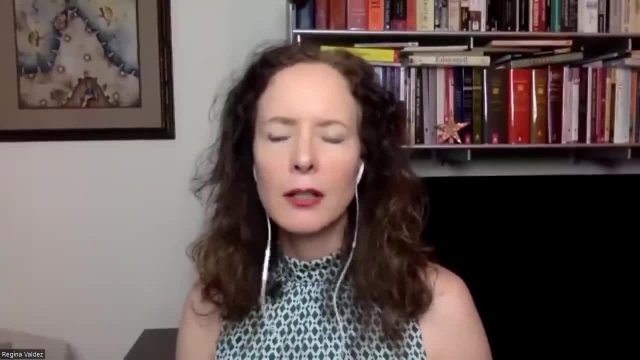 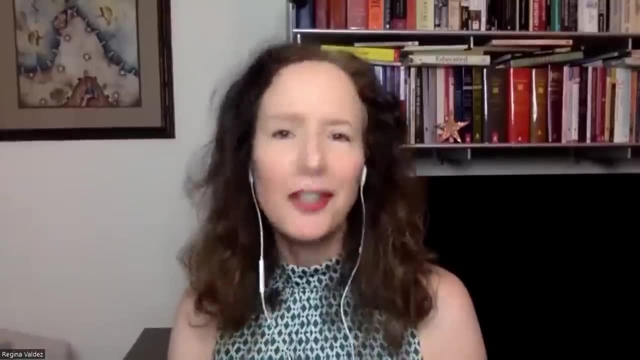 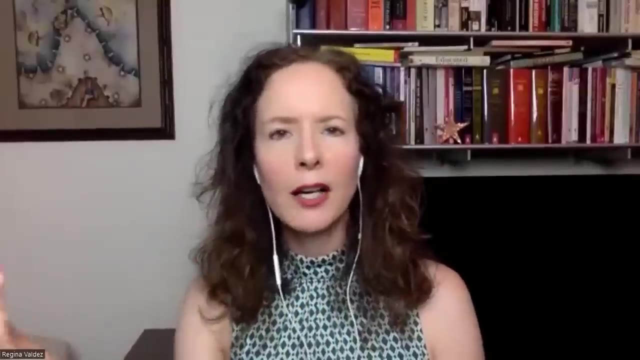 So if you think about it that way, it's really not so hard. Think about it: when you're in a room and it gets too warm, You want to turn on the AC. hopefully not too often. Maybe you turn on a ceiling fan to cool. So that again is a turning from one to the other When it's too hot. 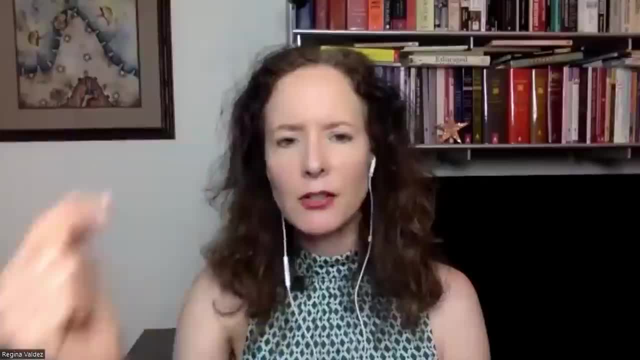 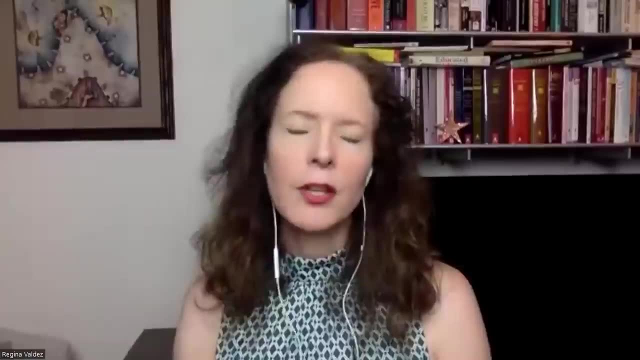 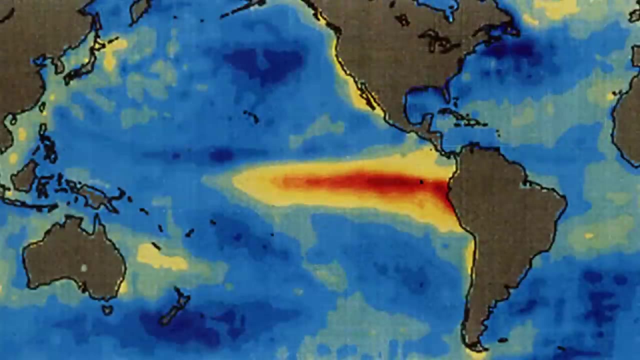 you want to move towards cold and then it gets too cold and then you turn the air off. So those are how they're described And they basically go back and forth depending upon the currents of the trade, winds and the upwelling of the water. So we're thinking of the warm water on 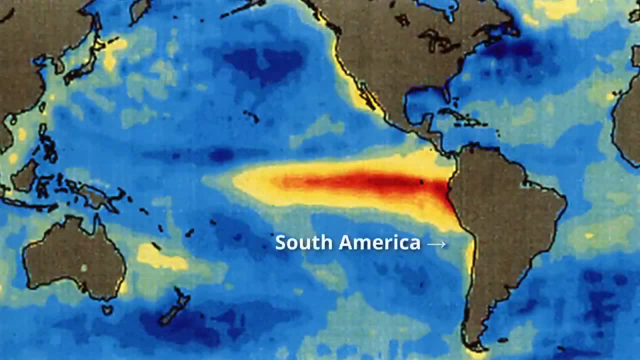 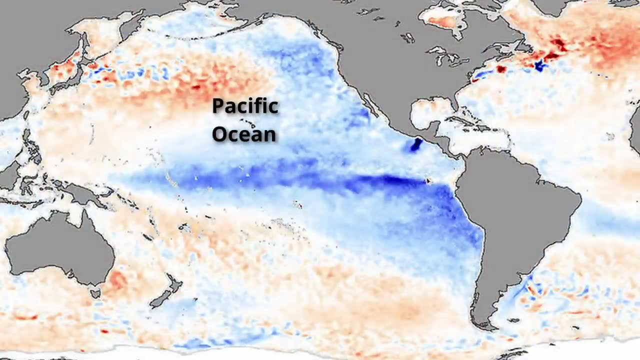 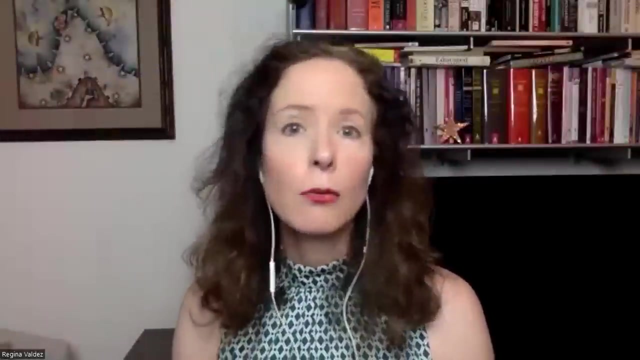 the north and southern part of the coast of North and South America and the Pacific Ocean, And the opposite is the same with La Nina, And each of them create their own weather patterns: Hot weather, cooler weather, rainy weather, drought and with climate change. 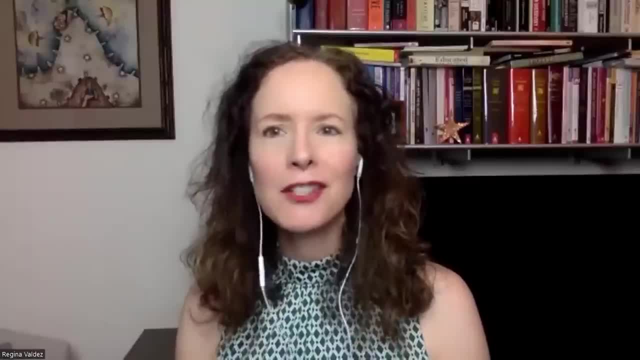 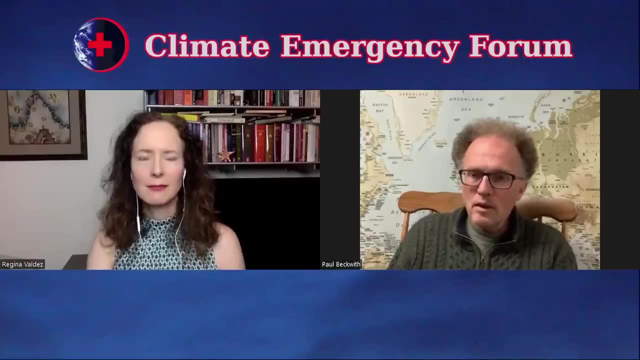 these are getting more extreme And I'm hoping, Paul, that you can take it from there and explain it to us in much more detail. Yes, thank you, Regina. So the term ENSO, E-N-S-O stands for El porte Nato. 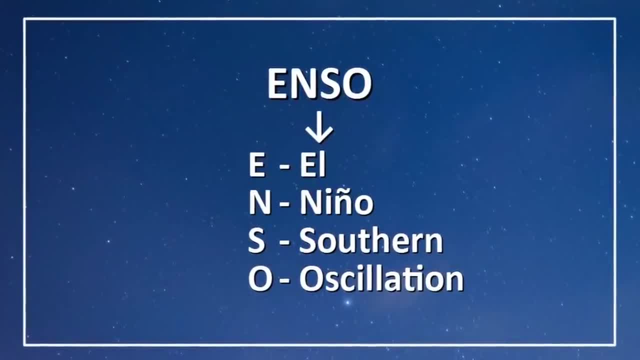 Southern Oscillation. So the Elejango part is really an atmospheric phenomena and the Southern Oscillation saying El Nino, much like the, The other parametric, 260 Gothes leave families, women, women of color in South America and for the women all. 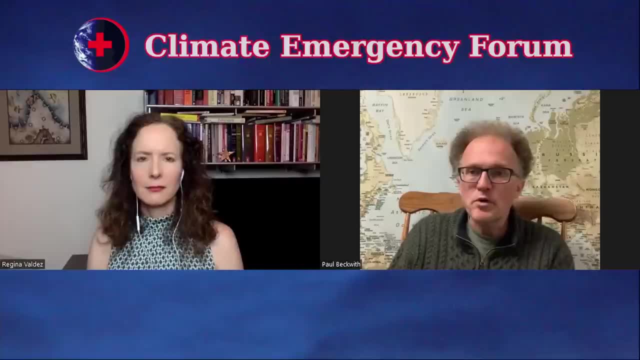 southern os Navy, but in fact Al Nino Highness is really one of the most African speaking Aboriginal peoples and a classic for the women of color, And this one property that creates an uplifting atmosphere that brings theanswhere to children. oscillation is the response of the ocean, but basically this is an ocean driven event, i think. 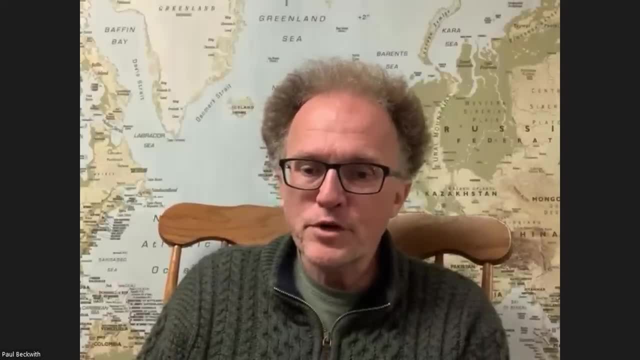 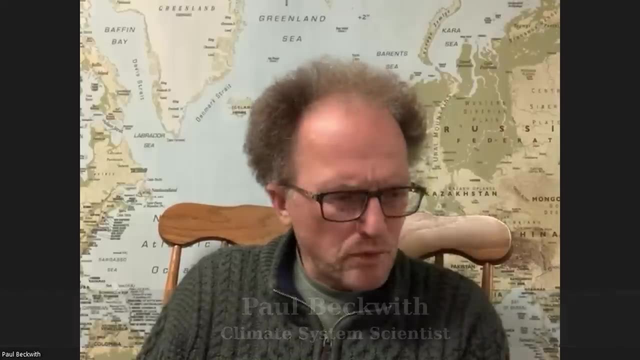 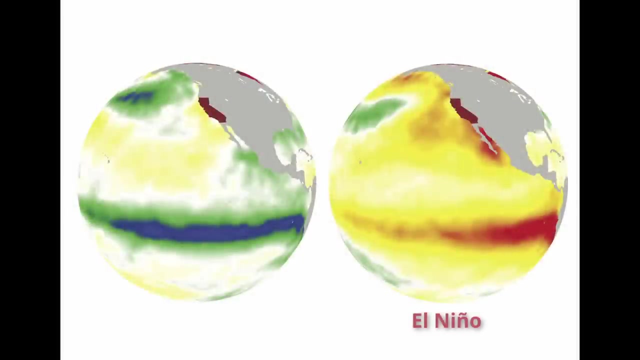 is most likely the ocean triggers it. we don't know for sure. it's a, it's a quasi periodic cycle. quasi because it's not. you know, there's a lot of variability in the period, so we're talking about anywhere from two to seven years. generally, after there's a strong el nino, then there will be a. la nina and then another el nino. it normally cycles back and forth, but not always. it seems that under abrupt climate change, with the greatly warming oceans and stratification of the oceans, that the behavior of the el nino southern oscillation or the enso pattern is becoming. 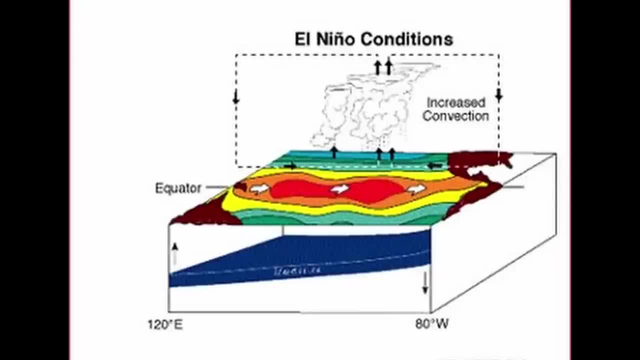 a bit more erratic. basically what happens is warm water on the western equatorial pacific pools and that warm water creates a lot of water vapor in the air and a lot of convection, and the air rises over the west pacific, at the equator, and then that air that rises spreads to 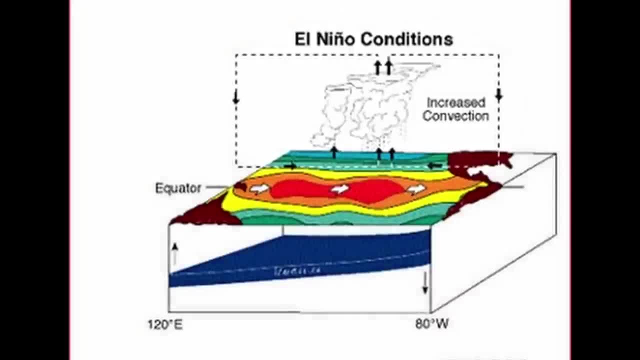 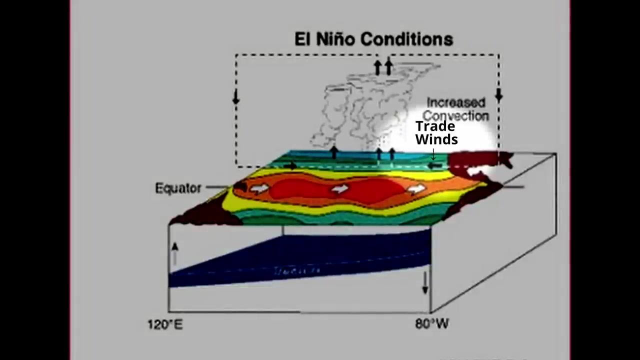 the east at elevation, cools down and descends over just off of the coast of south america. it descends down and it's and then, to complete the cycle, the winds then head to the west along the surface and we call those, uh, trade winds. quite often so those winds, when we have the warm ocean on the western pacific. 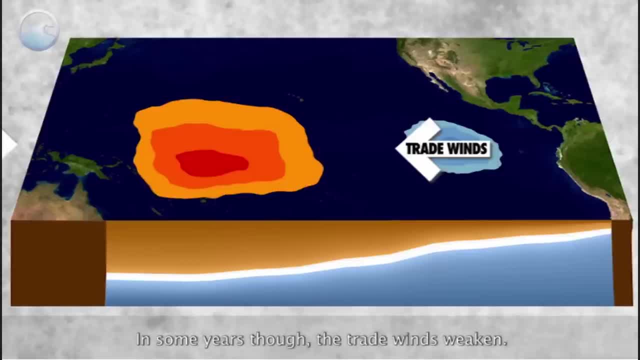 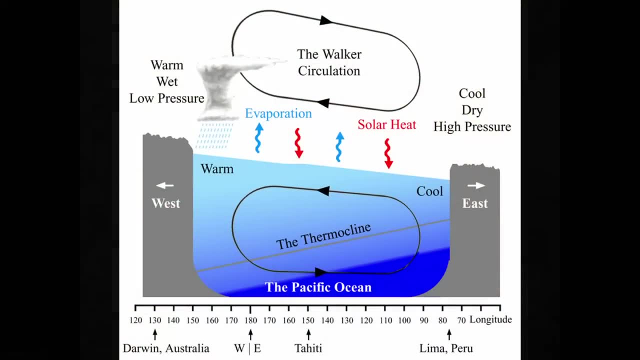 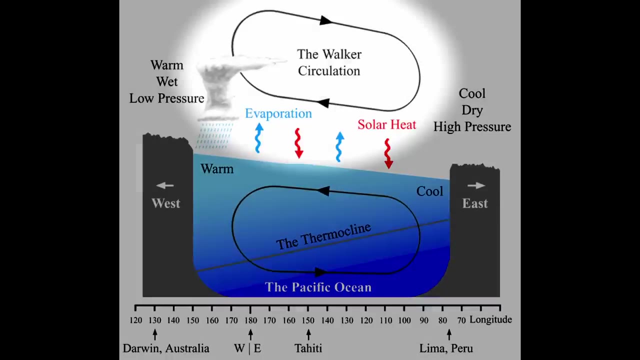 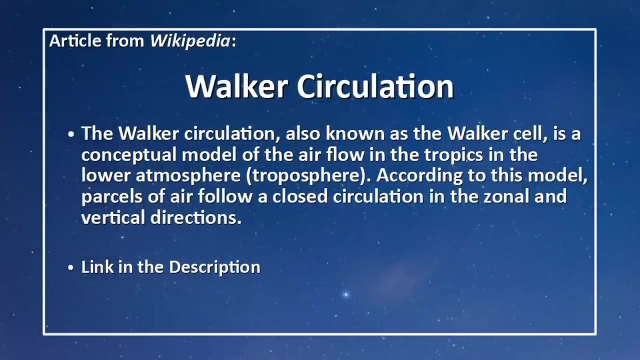 equatorial pacific will get cool water off south america because the water is pushed away from the continent and there's upwelling and that upwelling water is is colder, so that generally happens. that cycle is called walker circulation. now what happens when enough water- warm water- builds up in the western equatorial pacific? it once it's triggered and 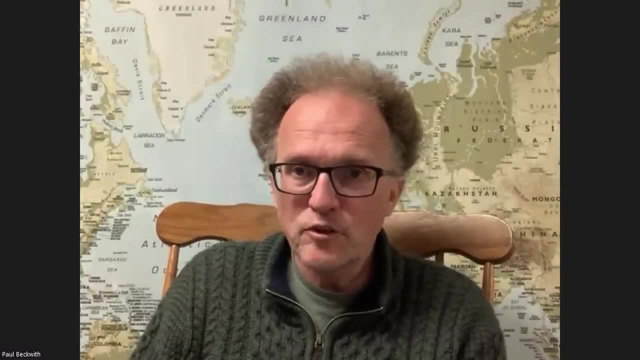 we're not exactly sure of the trigger. maybe it's just the huge, vast amount of warm water, not just at the surface of the ocean, giving high sea surface temperature, but over you know, to great depth as well, that warm water eventually builds up enough, and then it's. 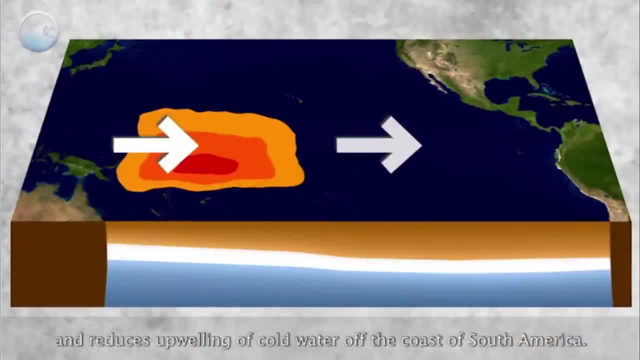 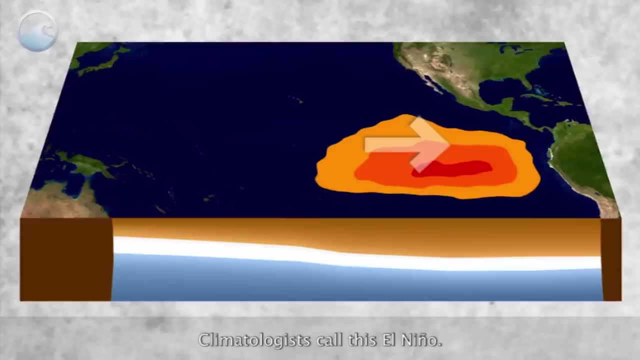 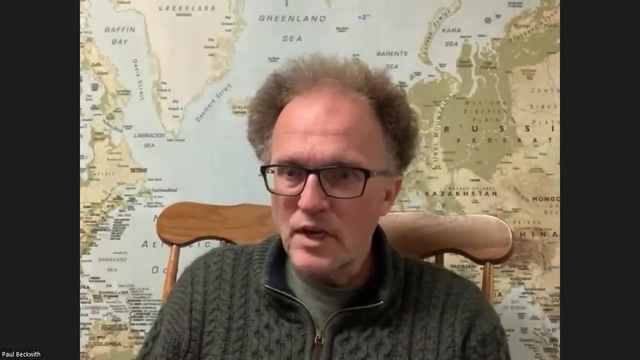 loshes eastward across the pacific until it makes it all the way to the coast of south america, bringing very, very warm surface water and water at depth. then what happens is you don't get that. the walker circulation greatly slows down because you don't have all that convective. 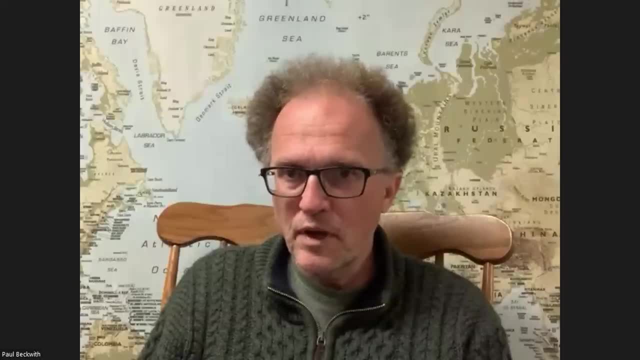 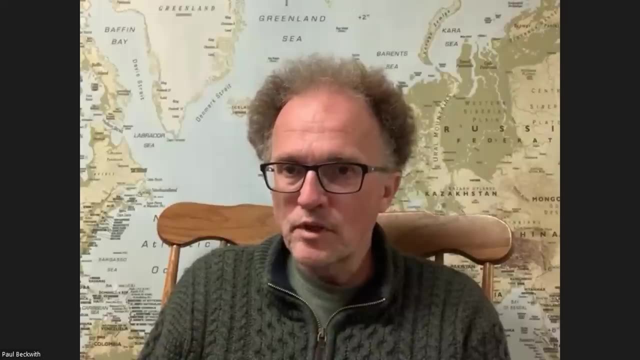 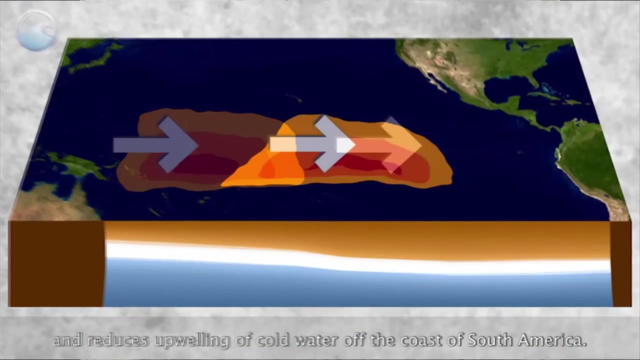 uplift on the western pacific. so that means that because the walker circulation slows down, the trade winds really really slow down and they're no longer pushing that warm water to the west so it can come right across the equatorial pacific and pile up off south america. 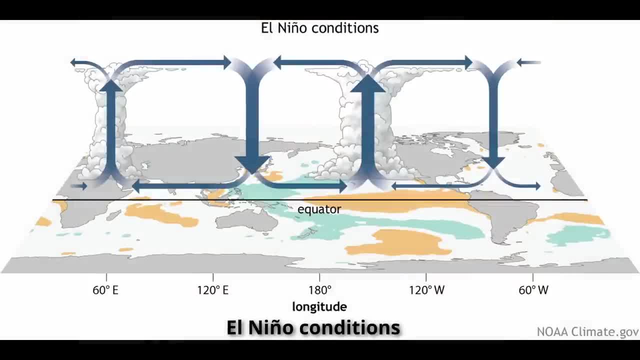 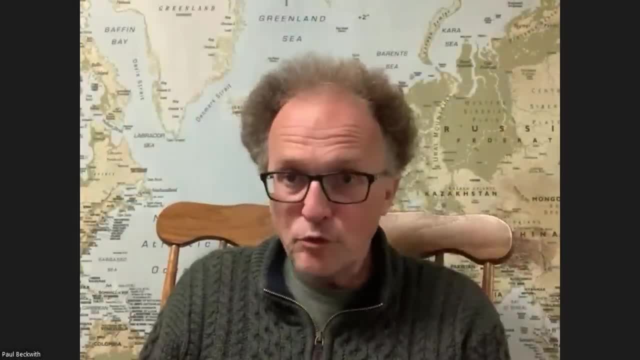 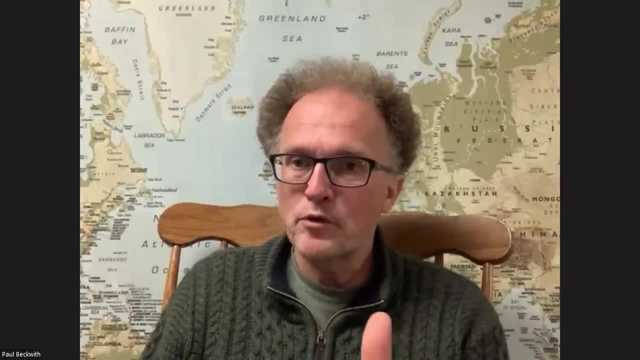 and that's the very powerful el nino phase. then, when the system re-establishes itself after the heat is released from the ocean to the atmosphere, that's the biggest thing. so we set global temperature records in the atmosphere when there's very powerful el ninos, because the global average temperature in the atmosphere can 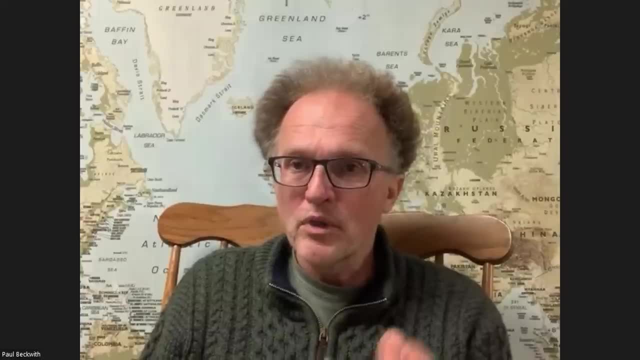 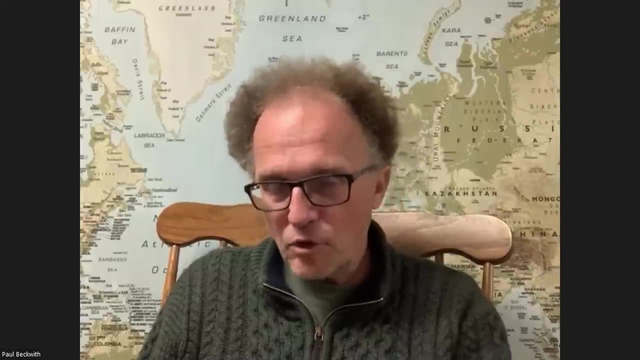 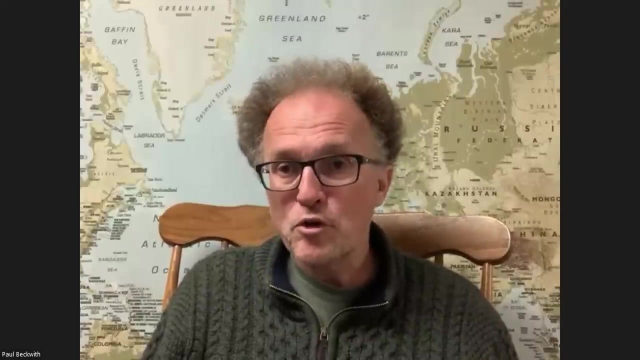 be 0.3, 0.4 degrees warmer than it would be without the el nino then. so after that energy is released from the ocean, then the cycle repeats, the warm water starts building up again in the west pacific. we can sometimes go to just a neutral state and not have, and not have the la nina appear at all. 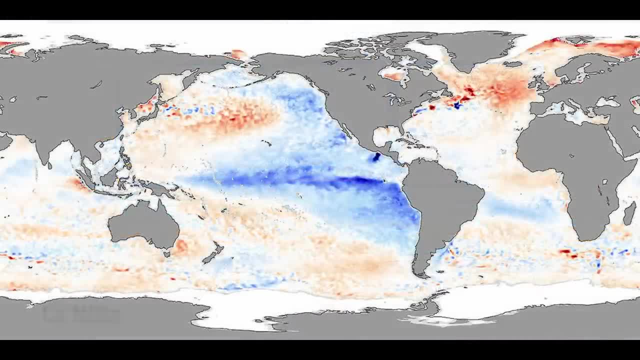 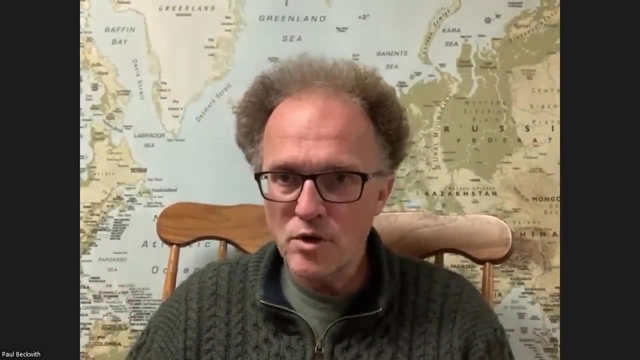 but generally the the la nina doesn't appear and then the equatorial pacific to south america is very cold, so obviously this affects the where heat is released and absorbed on the surface of the planet. we know over 93 percent of heat is absorbed into the oceans and, like i said, the ocean surface warming and we know that the ocean currents. 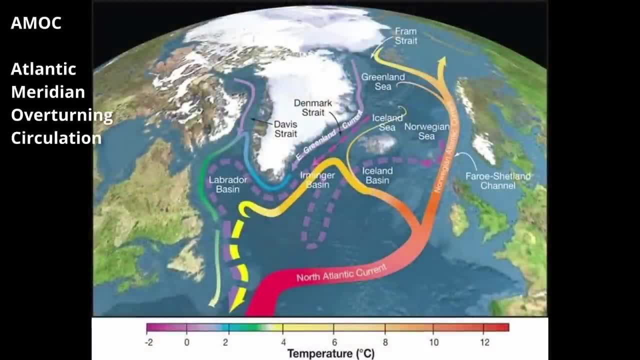 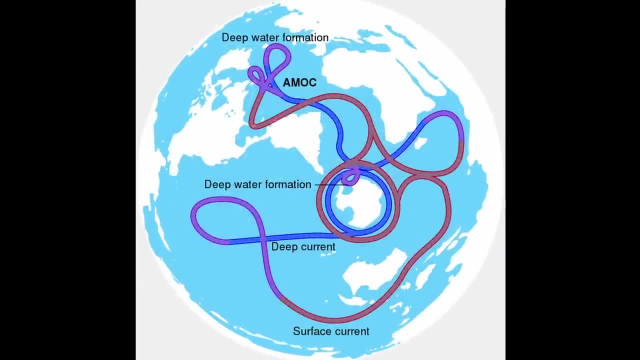 are also changing. i talked about the amok, the, the atlantic brindle, overturning circulation pattern. so the ocean currents are changing and the ocean currents are changing and the ocean currents are changing. the oceans are warming, they're becoming more stratified and these things seem to be having. 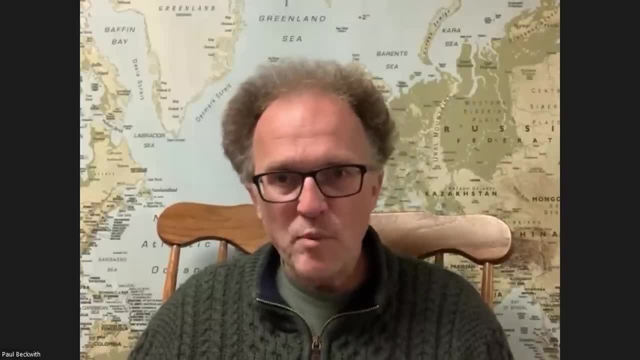 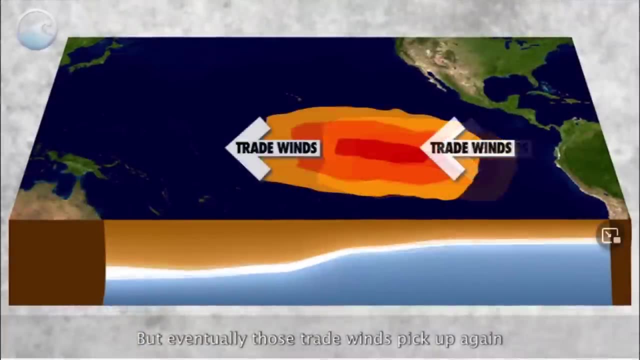 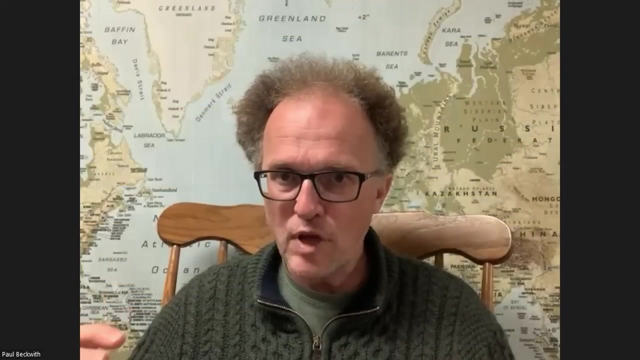 an effect on this cycle and we might- some people think we might- head into a perpetual el nino-like state. but what is interesting is the last several years we've had a very powerful la nina. okay, so if you go on earth- null school- and just look at the sea surface temperature and all the anomaly in the pacific ocean. you see very cold water extending up the planet. in the sea surface temperature it's much colder than what it used to be, but in fact it's much colder than what it used to be. now it's like cold in the middle of the east pacific. the area's very cold as soon as the water is out. the 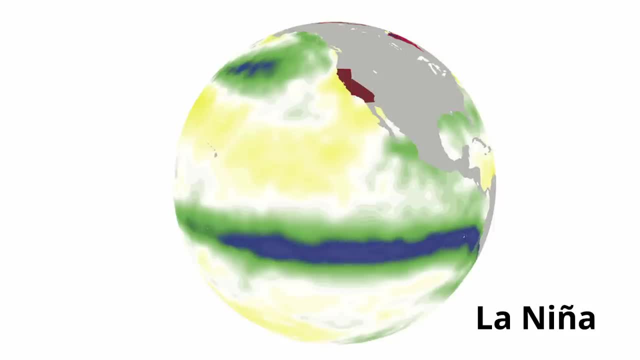 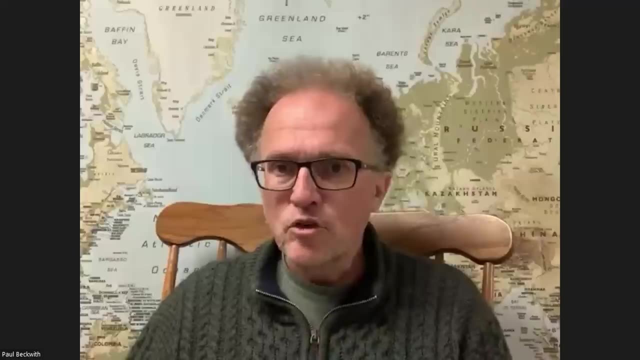 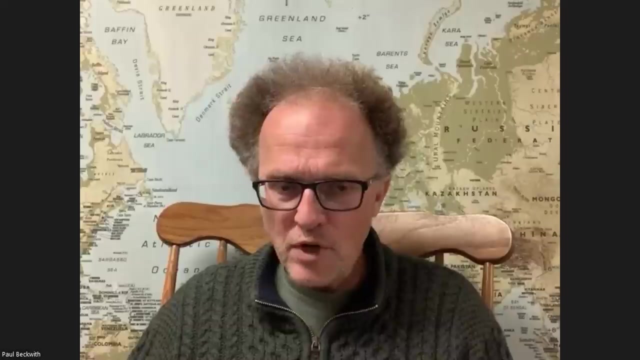 all the way to South America. so this is ongoing. it's been. it's been several years now that we've had this state, which is very unusual. it could set a record length. so you know there's a lot of interesting research that needs to be done to connect this more, to figure out the details and 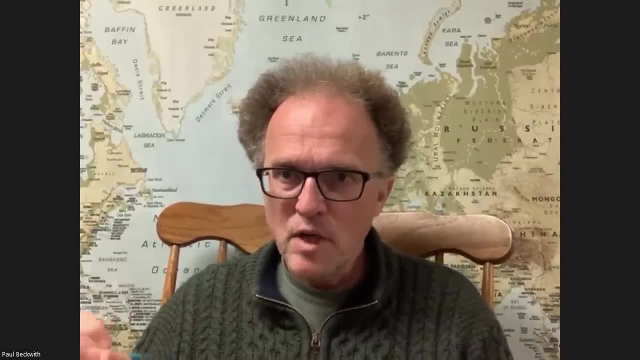 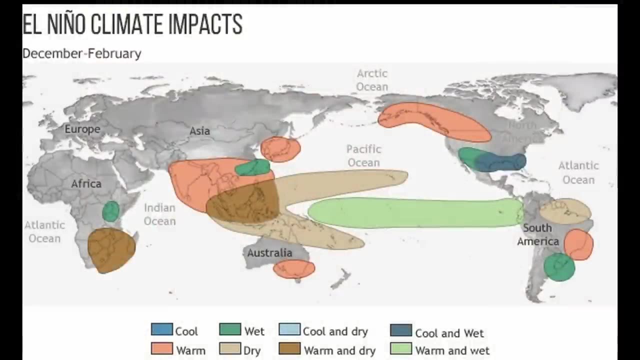 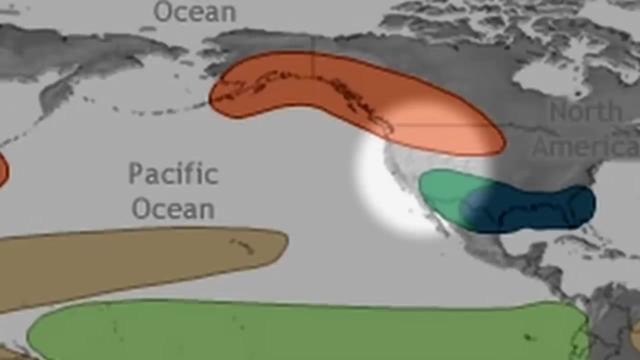 how it relates to the abrupt climate system change, but it's definitely. it definitely has global effects on rainfall, heat and drought around the planet. so, for example, you know, if you're in California and there's a strong El Nino, you generally get very, very heavy rains and landslides. 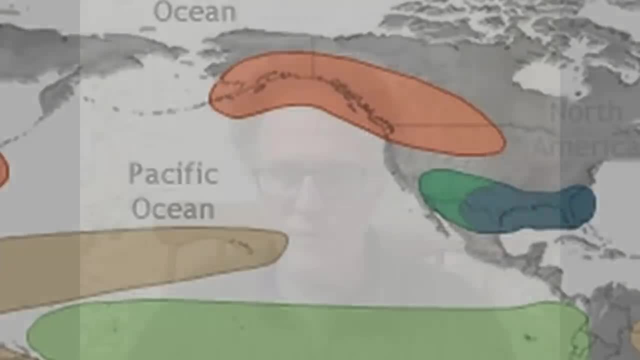 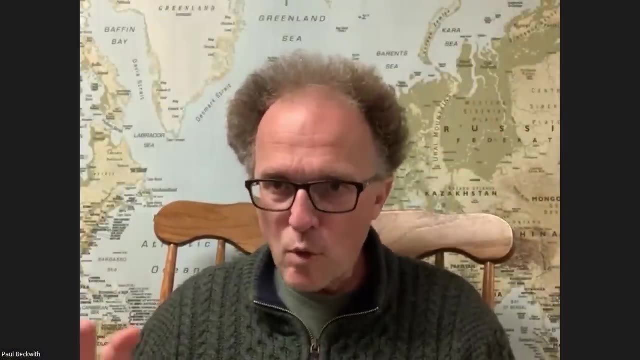 mudslides on the west coast of California. if you're on the east coast and there's a land, an El Nino, you get more hurricanes, so so you need to look at the global maps of where you are to see the effects on your location. but, in general, the El Nino's 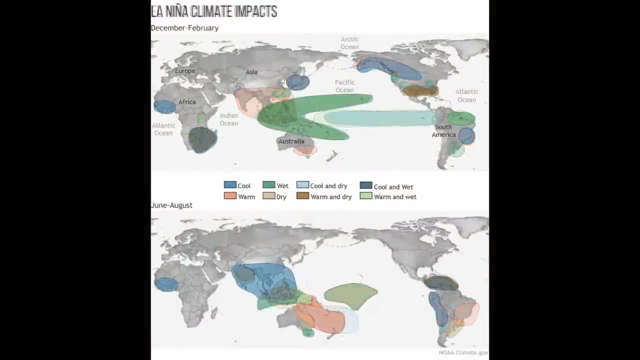 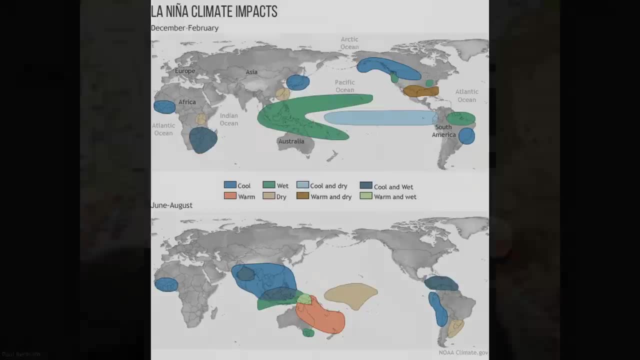 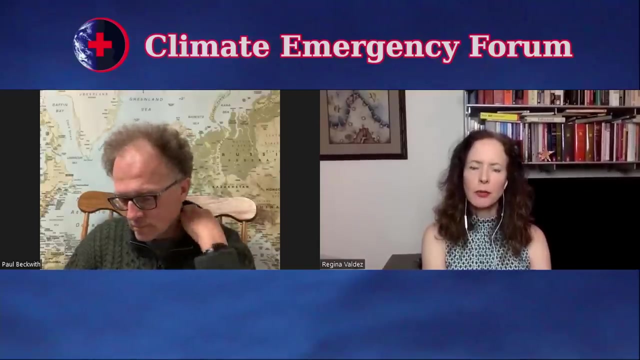 are about up to 0.3 degrees warmer than normal, and the La Ninas can be the opposite, cooler than normal. and that's on top of the climate change warming. Thank you for helping us understand that a bit more, Paul. I'm just just a quick question because I want to hear what Peter has to say. but 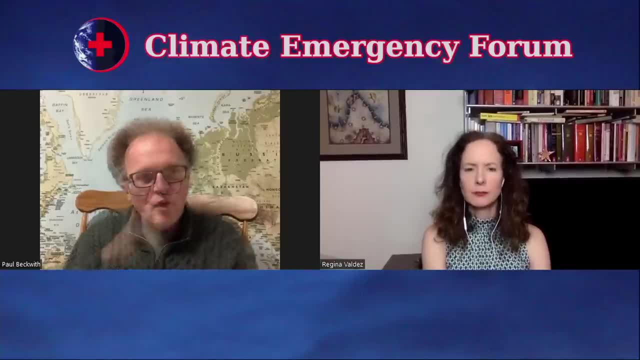 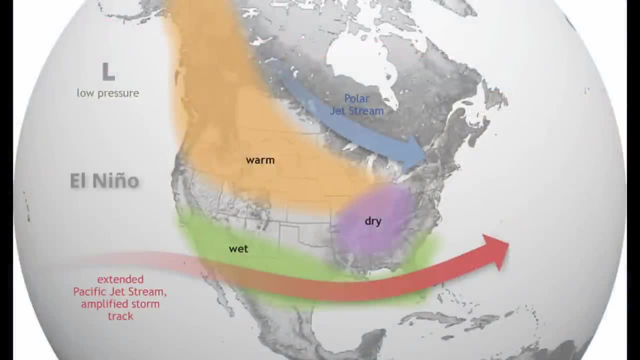 just. is El Nino more problematic for us than La Nina In the northern hemisphere? generally really depends on where you are, but we generally think of El Nino leading to more extreme weather conditions, more torrential rains, places leading to flooding and lots of damages, say. 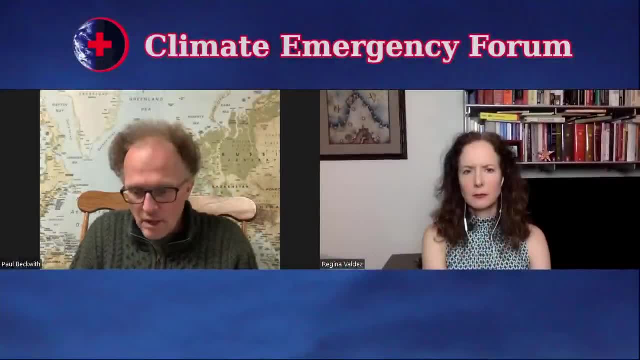 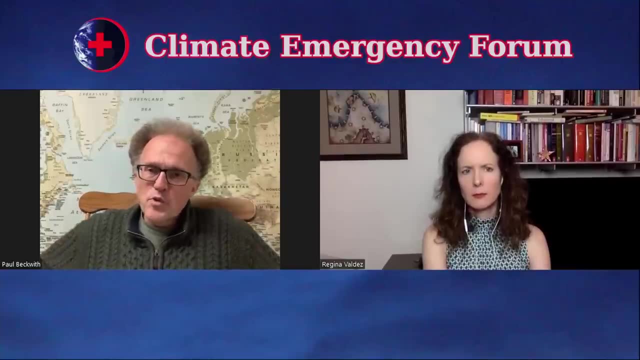 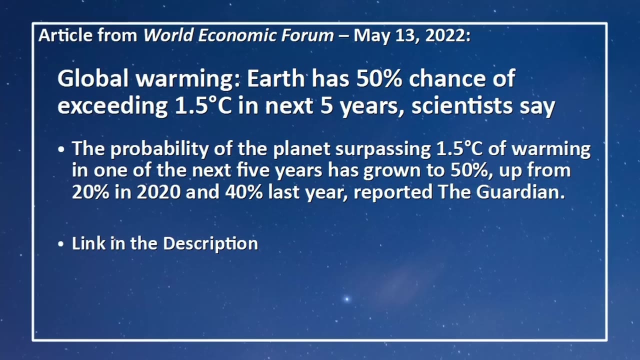 you know, also in the southern hemisphere generally La Nina is a tamer sort of thing. El Nino is is a big factor and you probably are familiar with the report saying that you know the chance is 50 percent that will break the 1.5 degrees celsius guard band in temperature and 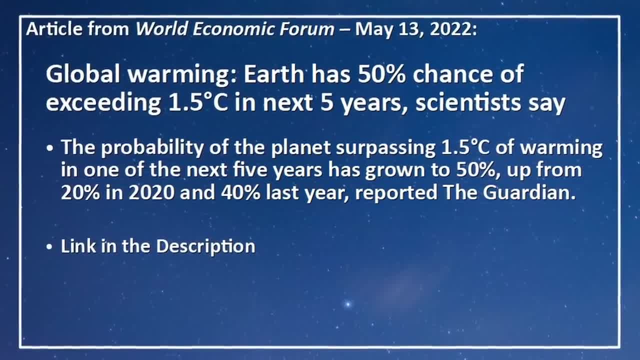 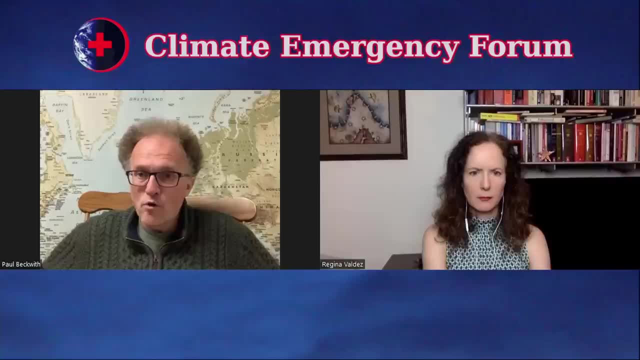 next five years and that will push us globally over the 1.5 for the entire year. In past El Nino's it's pushed us over the 1.5 for a month at a time. Generally the- you know, February, March months have reached those sort of temperatures 1.5 and again, depends on what baseline you use. They 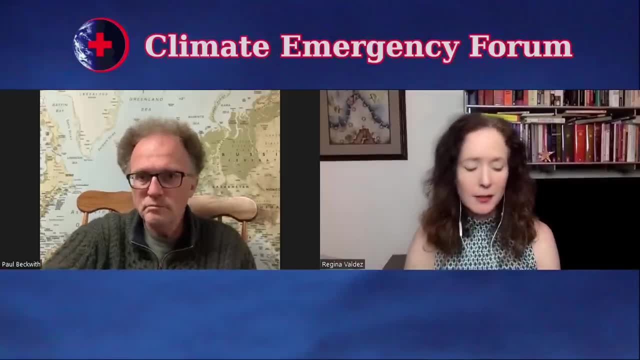 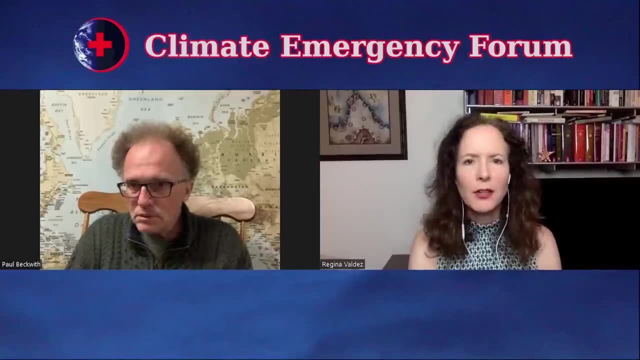 Wow, Yes, I did read that. I'm sure most of people watching have read that- about us surpassing the 1.5.. I know this is a topic that's near and dear to Peter's heart and, Peter, I'd like to hear what you have to say about El Nino and its effect on the planet and the climate, and 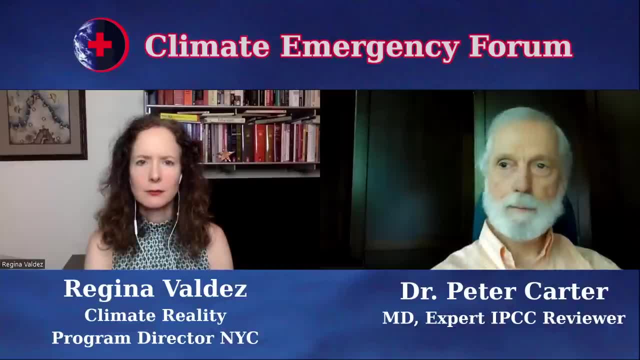 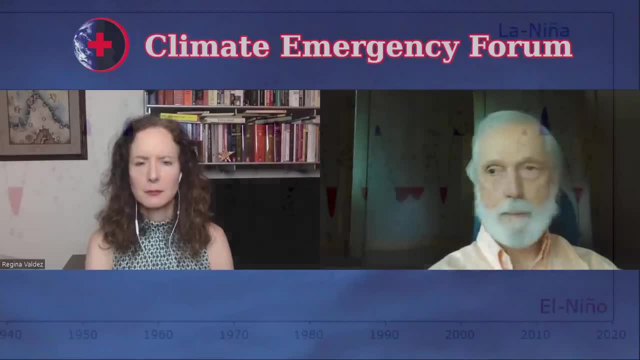 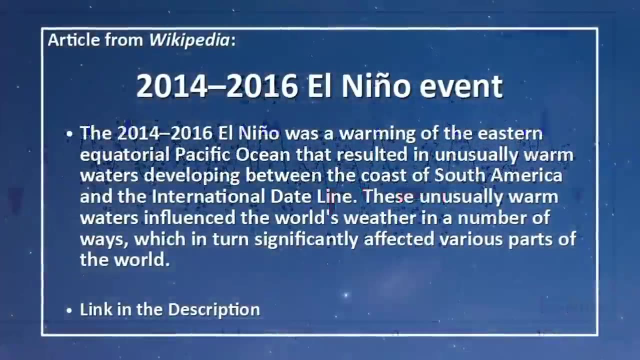 our oceans and our world. Thanks for you know, thanks for explaining the processes and systems so well, Paul. So the last big El Nino was deep in the mid-60s, It was the first big El Nino. that was 2015,, 2016,. and the southern hemisphere, the people, populations of the southern hemisphere. 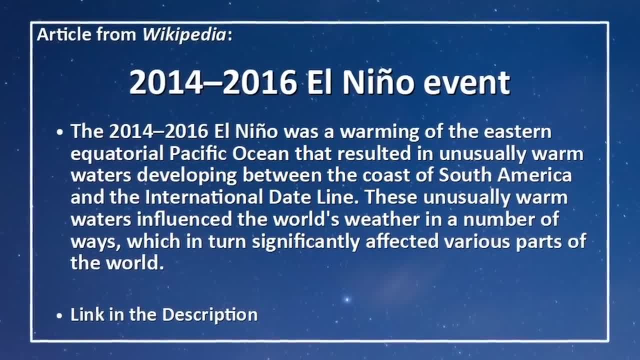 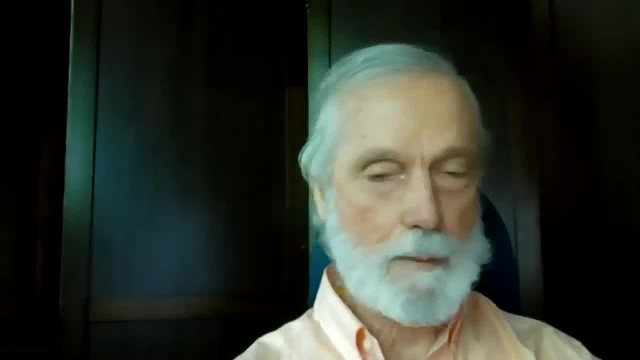 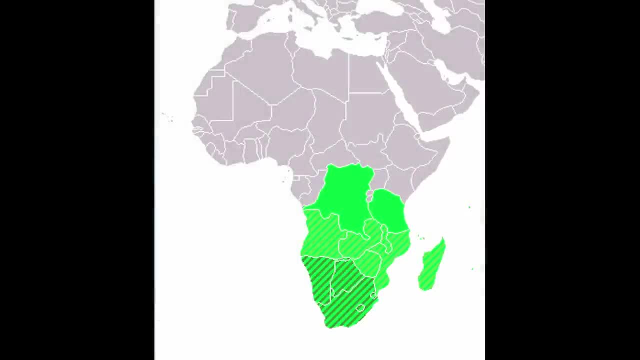 were hammered severely. As Paul mentioned, there's increased flooding in western North America and some increased heat in various regions, but in the southern hemisphere a huge region of southern Africa was hit by drought and heat. India and Pakistan were hit by drought and heat. 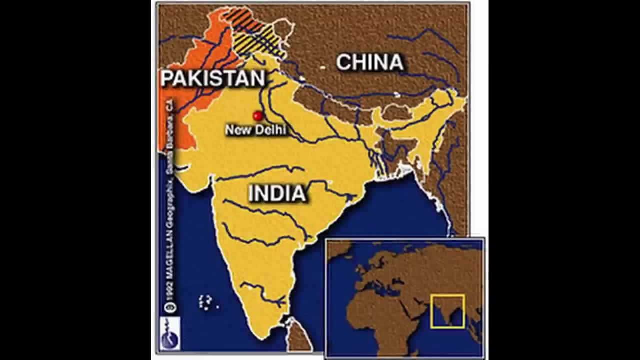 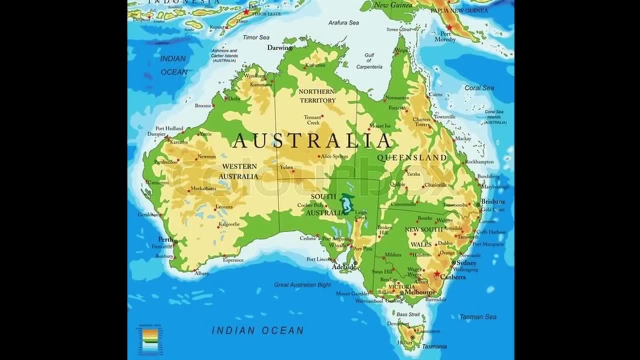 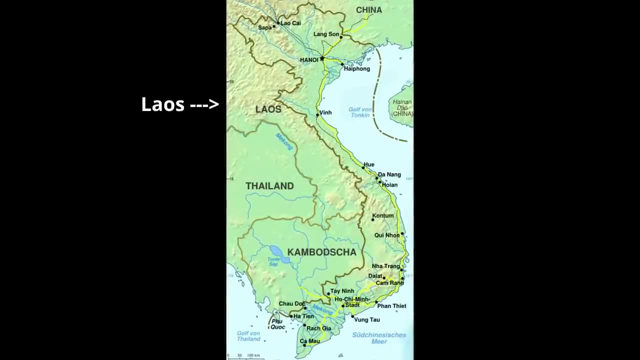 Just imagine that they're there right now. What is actually their maximum summer? They have unprecedented heat and unprecedented drought as well. Australia was hit by heat and drought. Vietnam, Laos- those regions were also hit by heat and drought. So the impacts on the southern 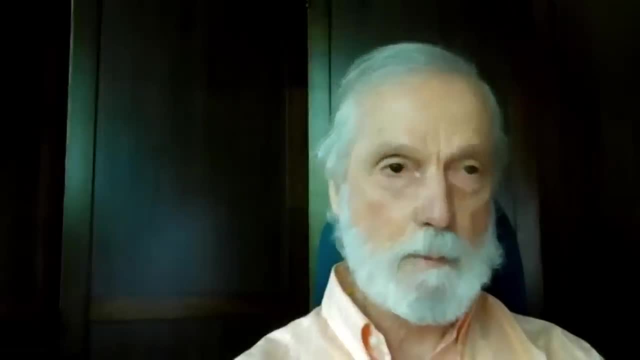 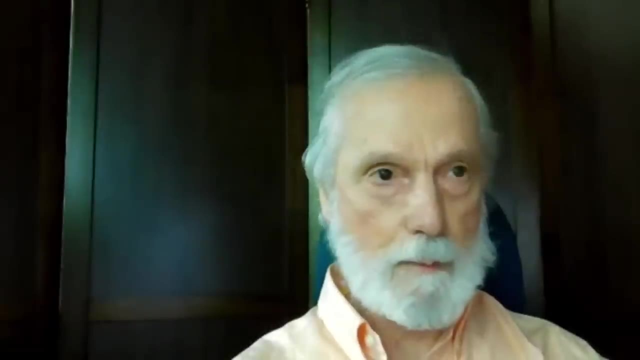 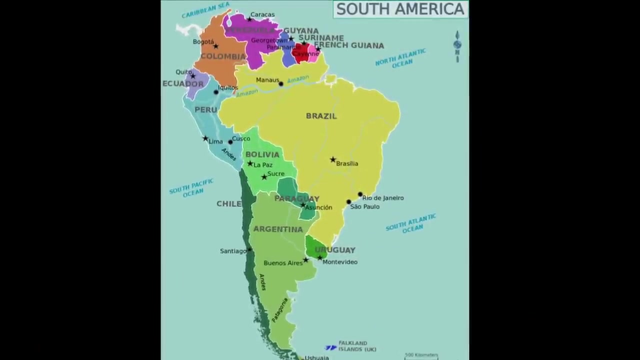 hemisphere were vast and wide. These are huge, huge geographical regions in which the temperature was altered severely. And then, Paul's already mentioned, there was increased flooding in southern South America, but in northern central South America, again, there was drought and heat. 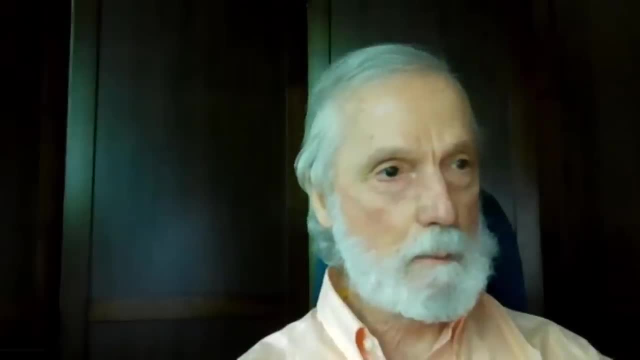 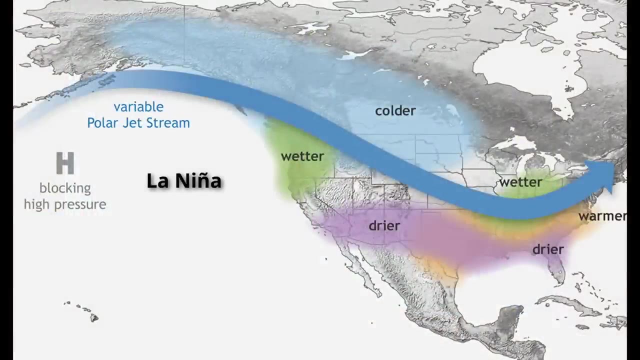 So we really should be afraid of the fact that global surface temperature is increasing rapidly. We should also be very apprehensive of the fact that, although we've been in this cooling La Nina for three years, we are still at 1.2 degrees C. That's the global temperature increase, which is big, big, big And so 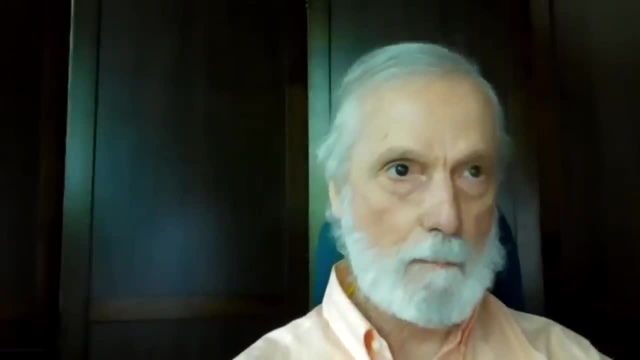 we're going to be at 1.5 by 2030.. So imagine another big El Nino like 2015-16, on top of a rapidly increasing global temperature. We're going to see unimaginable catastrophes across, presumably the southern hemisphere. So we're going to be at 1.5 by 2030.. So imagine another big El Nino like 2015-16, on top of a rapidly increasing global temperature. Vast regions, huge populations, 60 million people in 2015-16 were impacted severely with regards to. 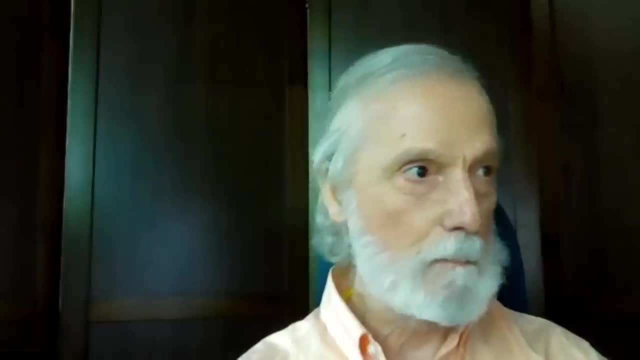 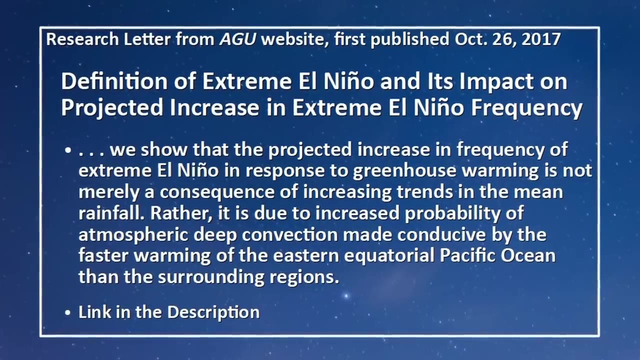 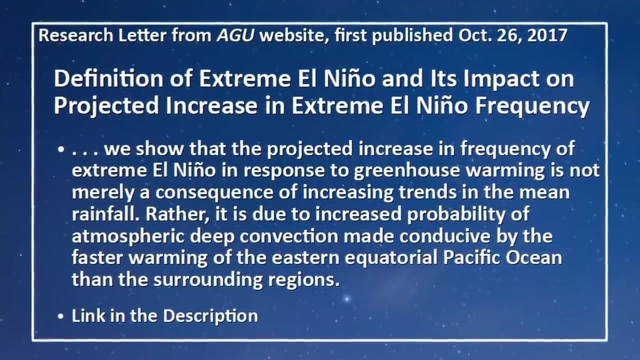 their food and water security. A lot, a lot of suffering. I want to mention some recent research. The most important research that I can remember came out in 2017. And that found that, under a likely emission scenario in which we're on. 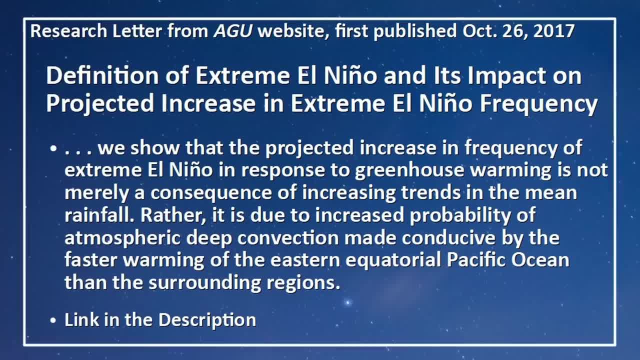 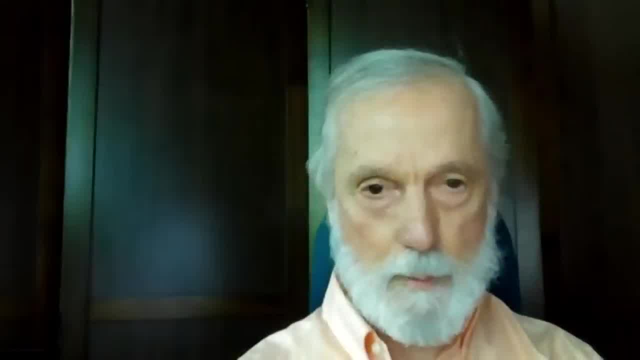 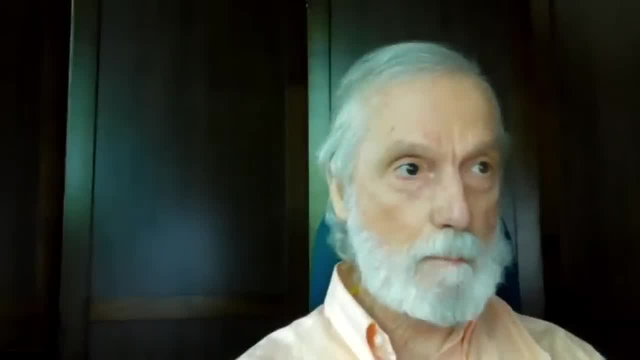 el nino frequency will increase along with global warming. so all the time we're increasing the global warming, which we are by pouring out um greenhouse gas emissions, the frequency of el nino will uh will keep increasing and um their models projected that at 1.5 degrees c, the el 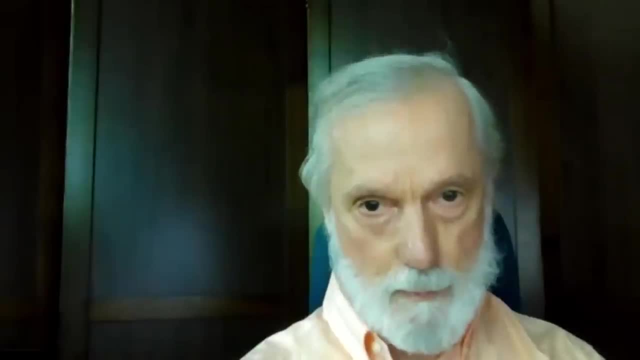 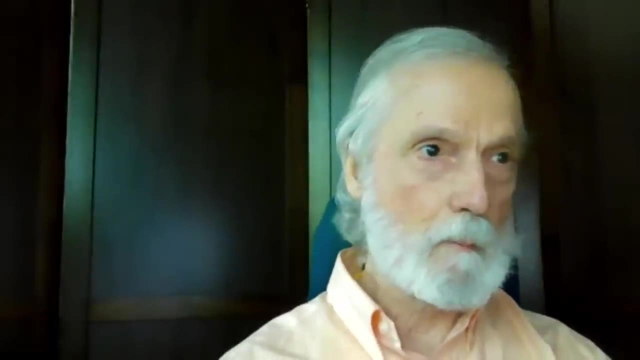 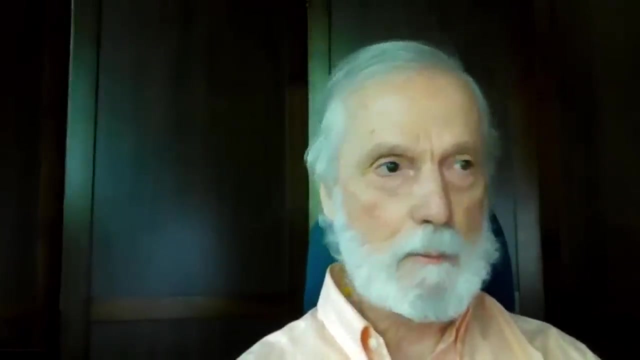 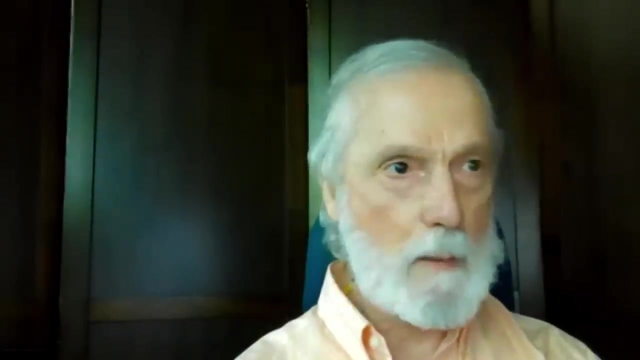 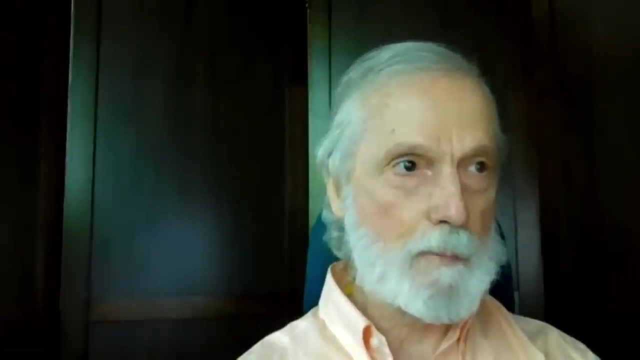 ninos will be double the frequency that we've been seeing, so that's absolutely huge. the thing that really uh interests me particularly is uh watching the global temperatures but also watching the atmospheric co2 concentration, and there we see absolutely sudden, dramatic changes. so the other big el nino was um 1998 or so and in both cases within a year um atmospheric co2 increase. jumped up the um. in 2013, the increase rate, the growth rate of atmospheric co2 in a year, was about um two parts per million. then in 2015 it jumped up to 2.95 parts per million. in 2016 it was over three parts. 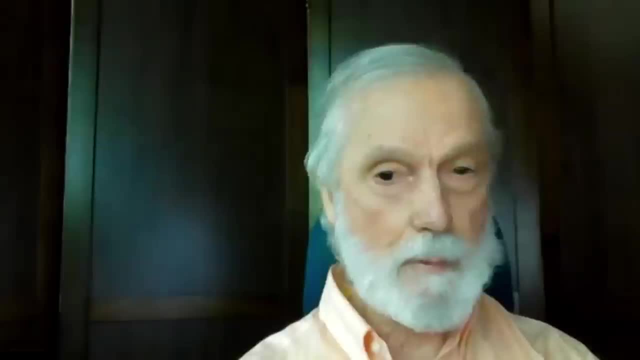 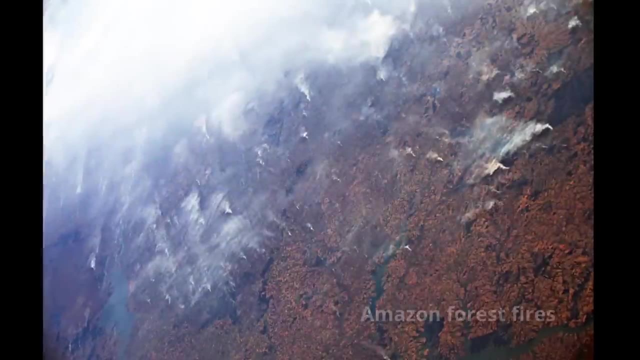 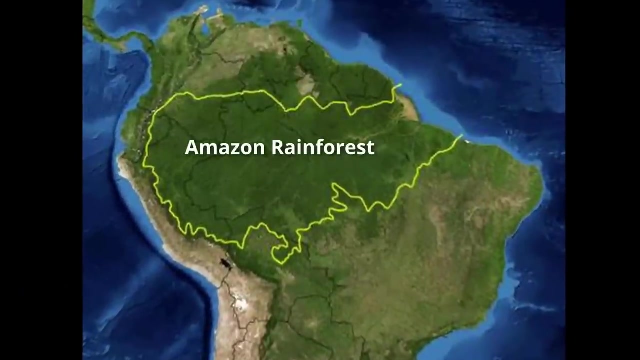 per million. that's a huge, huge increase in atmospheric co2 and that's attributable to the carbon cycle changes of the el nino and particularly widespread fires- and we've got fires bad enough already, so you can imagine what's going to happen with el nino and the amazon and the tropical rainforest, the um. the increase of temperature that paul's already mentioned that. that's really dramatic as well. it goes up by about 0.1 degrees c in a year with an el nino, so in a decade our global temperature is increasing at 0.2 degrees c. so we got this huge, huge, sudden jump in. global temperature as well. the record temperature um uh- global temperature increase- is still the 2015-16 el nino, and that was 1.3 degrees c, but the highest temperature ever recorded was recorded in march of 2016 at 1.66. 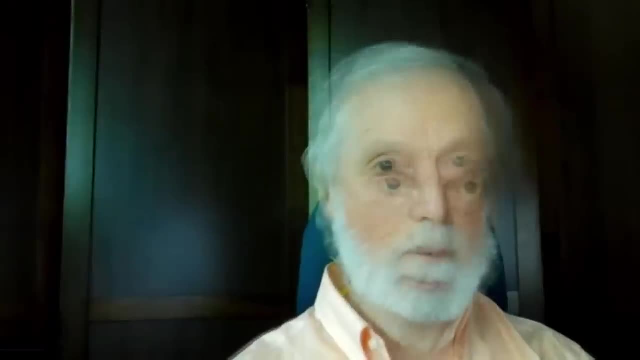 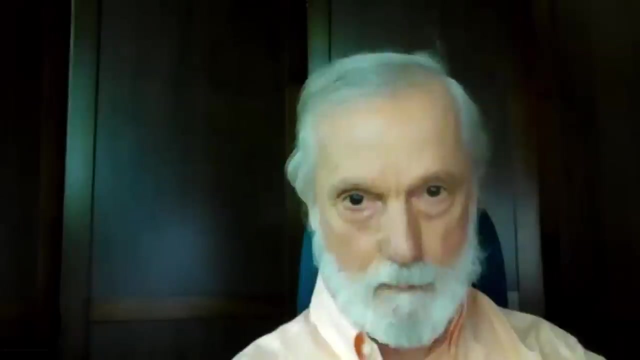 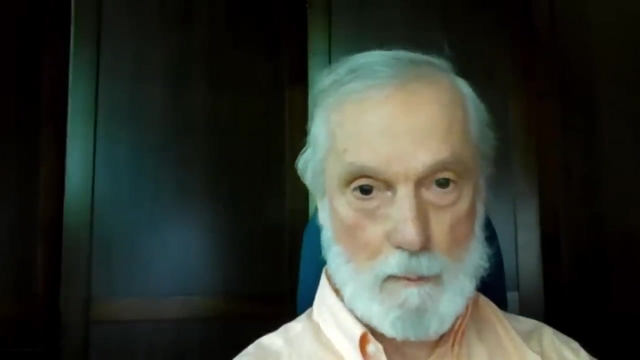 degrees c. so, as both regina and and paula mentioned, we're looking at a higher uh degree of warming very, very, very soon, very soon, and when this cooling dissipates, then we're going to be back up to an accelerating global temperature increase and it's truly terrifying to think that there's going to be. 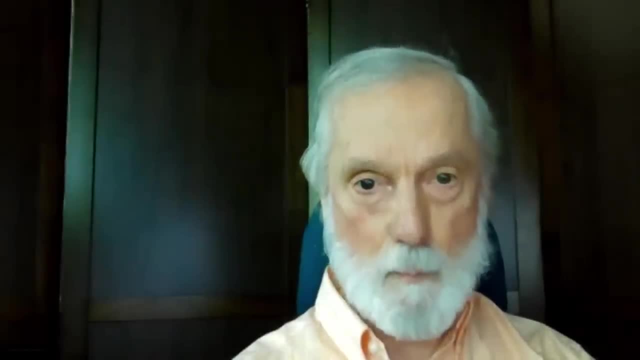 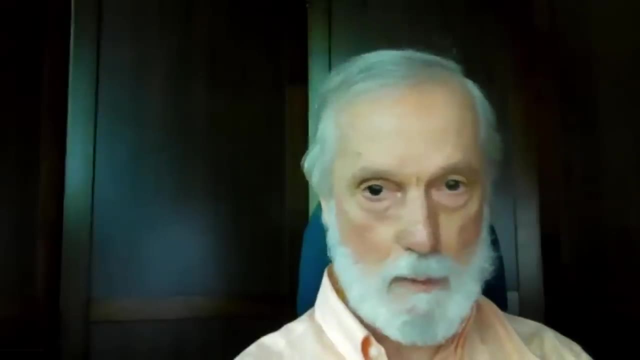 another very big el nino. um, it will be sheer hell, no question. 2015-2016 was horrible, absolutely horrible. so i i guess with that, i think we're going to have to wait and see what happens next. but, um, uh, dismal, thought i'll. i'll finish, thank you. thank you so much, peter, and thank you for. 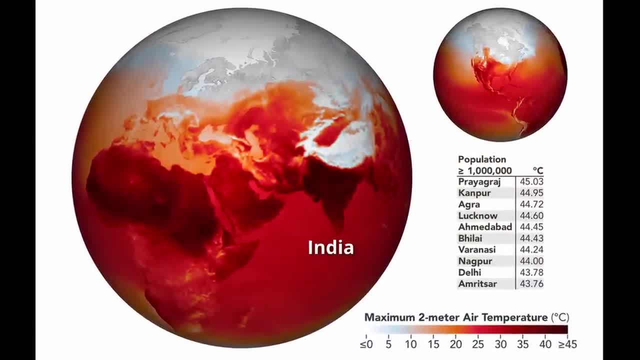 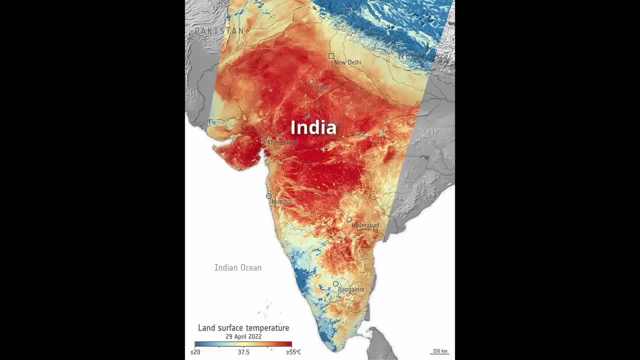 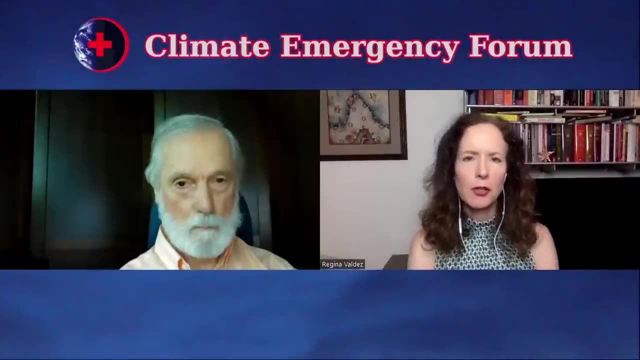 reminding us about the extreme heat that's going on in india and pakistan. it's really unbelievable and in and one way, it's kind of lucky, because apparently the wet bulb temperature kept the heat at a, at a level where there weren't massive deaths. um, i know that paul has spoken a lot about. 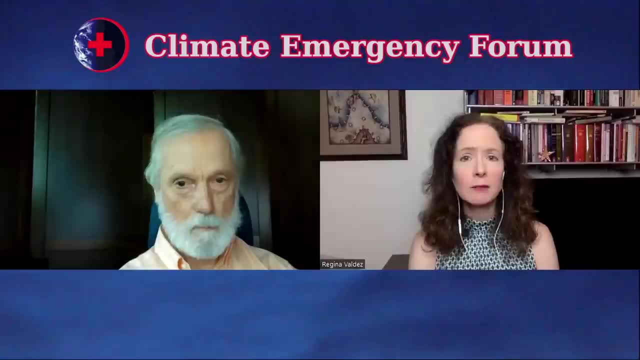 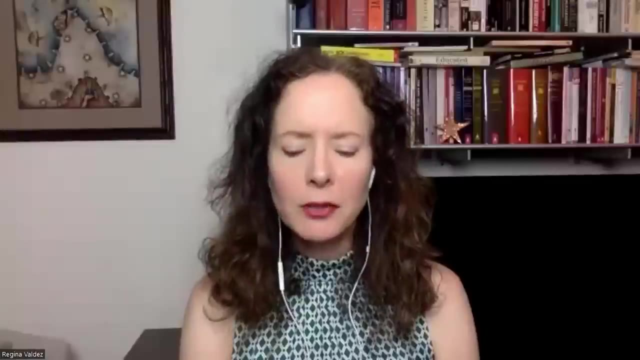 wet bulb, and that's something that that we'll probably be speaking out a lot more in the future, because it's going to be a very important thing for us to focus on in terms of survival- and i want to turn it back to you, paul- and this, uh, el nino la nina phenomenon. it's really amazing to me that. 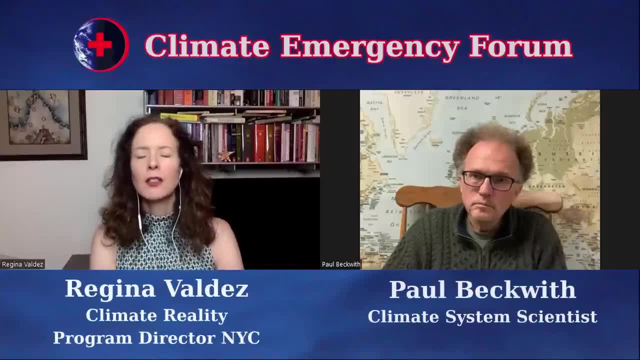 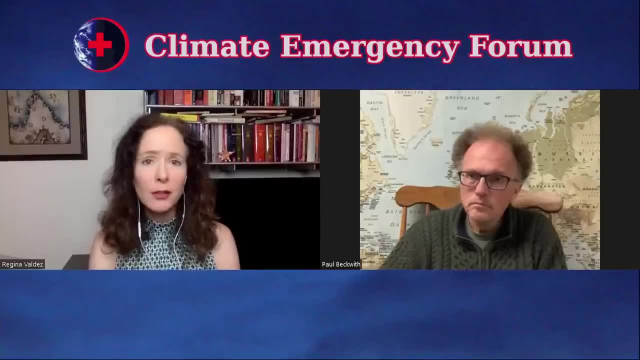 this is occurring in the pacific, but it affects us worldwide and you know, i think this is just a metaphor for how climate change and extreme weather doesn't just stay in one place, it's a worldwide thing. and one quick question i have is: are la nina and el nino in a dance together? in other words, do they coordinate? 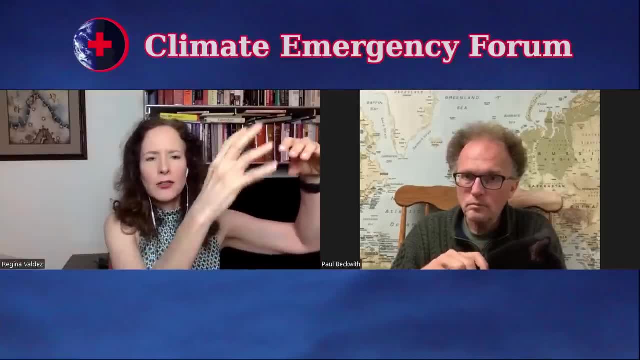 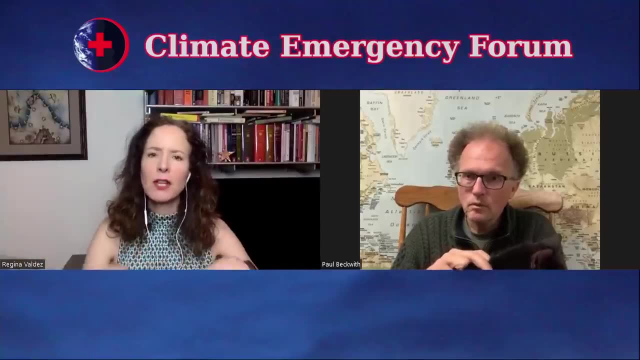 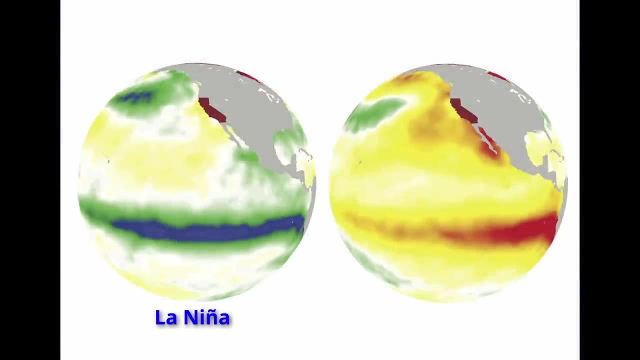 like when el nino goes this way, la nina goes that way and then the other way, or can it be whacked off balance? are they in tandem, so to speak? do they work off of each other, or can el nino just run wild? yes, so i've mentioned that. uh, you know, the general cycle is is anywhere from two to seven years. 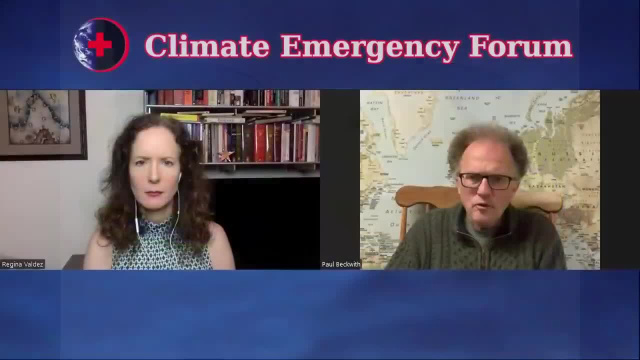 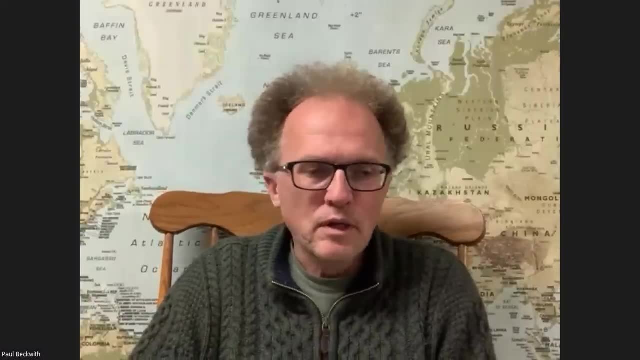 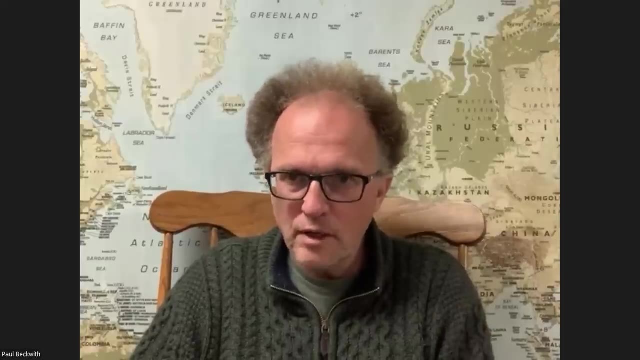 it's a quasi periodic, so somewhat periodic, so you can talk about it like a pendulum or an oscillator, but you'd have to say it's a complex pendulum. so in other words, instead of just a simple pendulum where you have a weight on a string, you have a string and then a weight and then from that. 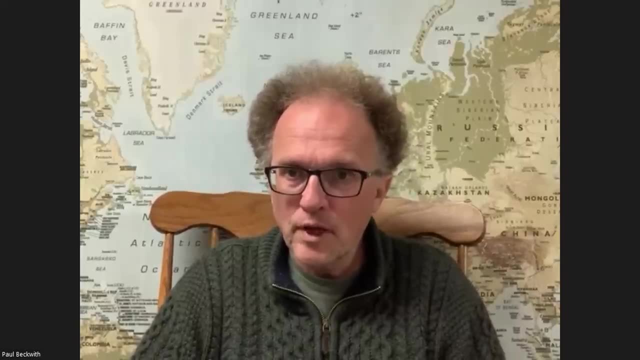 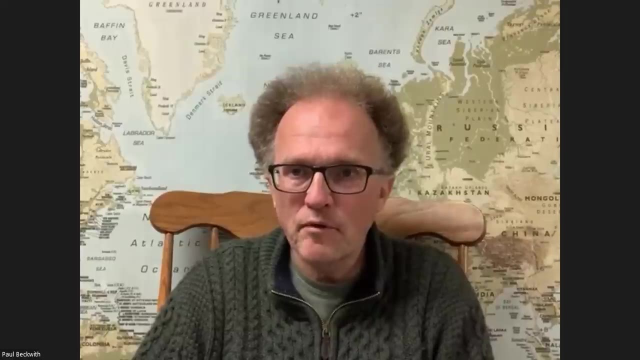 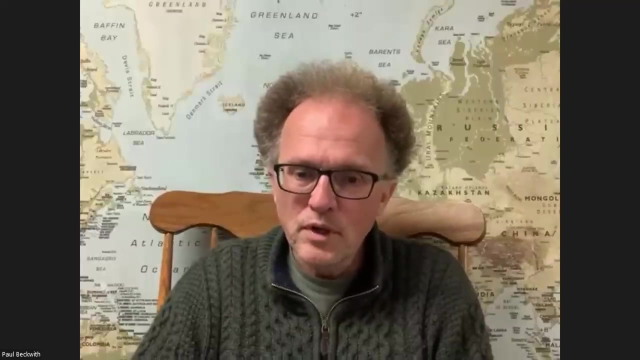 weight. you have another string to another weight, so it's it's a complex pendulum and it can can have nonlinear behavior and very unusual behavior that is difficult to model. so I would compare it more to that sort of thing because what we're finding, as Peter mentioned, with climate, 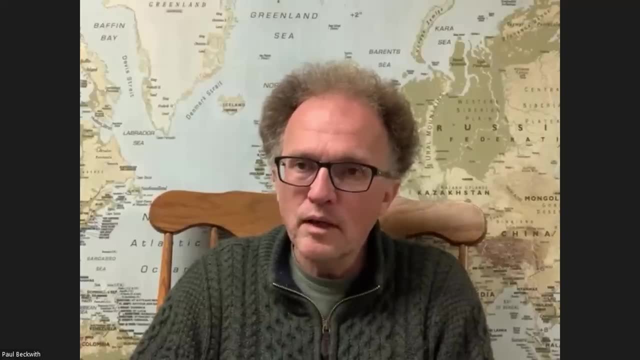 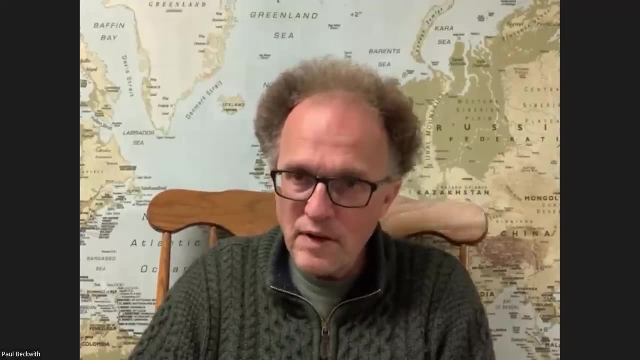 change, and some of the papers are indicating that we could become more or less stuck in the El Nino type phase and very rarely, if ever, get the La Nina cooling phase. so then the warming of the energy can be very, very powerful, but also the energy of the energy, energy conditions. 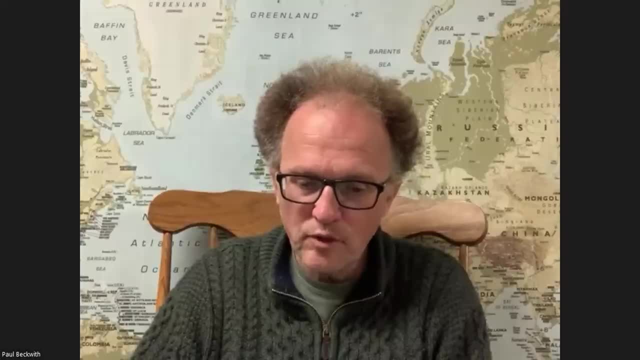 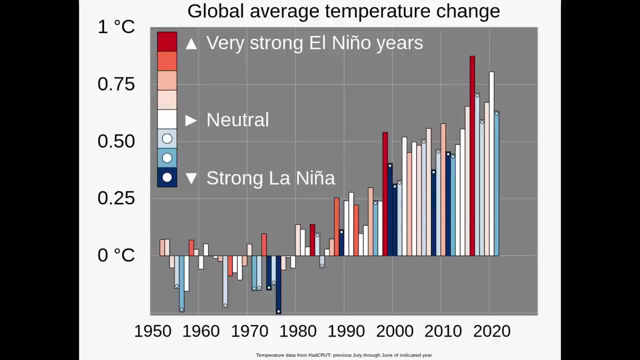 or the renewable energy, and the energy or the energy energy conditions can be very, veryíve, a little different, the planet will accelerate. Now a couple of things that very good points. that Peter mentioned is: when we have a strong El Nino, the global average temperature is higher. The ocean temperatures are. 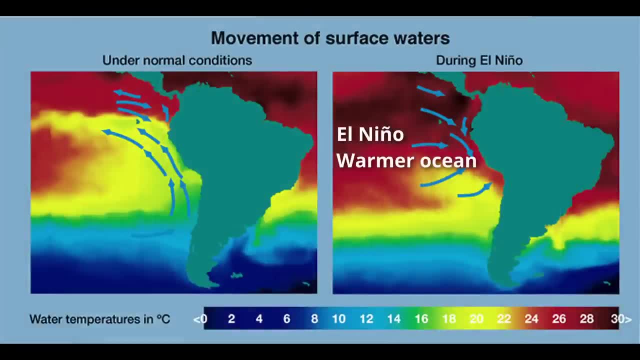 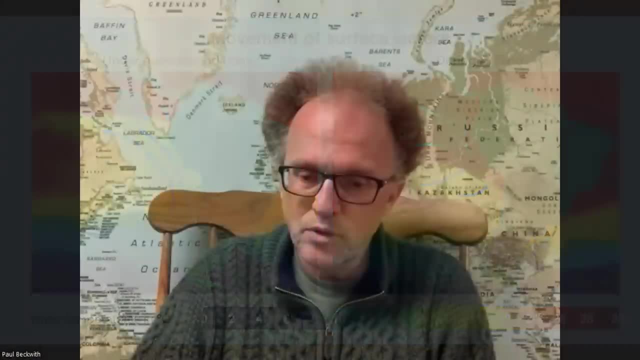 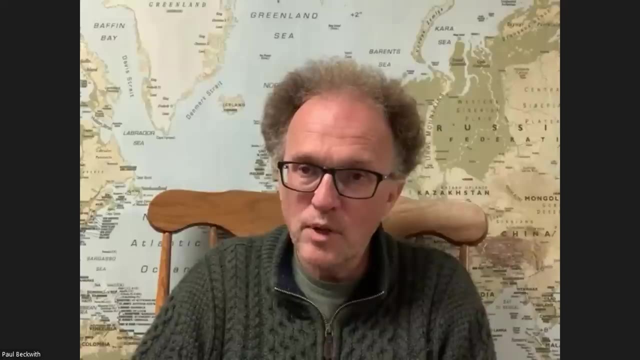 higher, And when the oceans are warm, their ability to dissolve gases is reduced, So a warm ocean cannot hold as much CO2.. So therefore, there's more in the atmosphere when we measure it, So that's why the rise was about three parts per million in 2015,- 2016,- when we had the last. 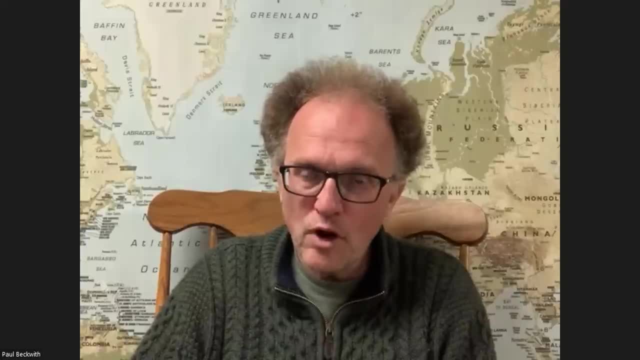 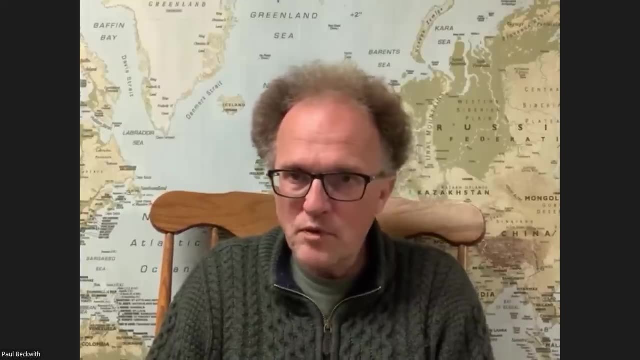 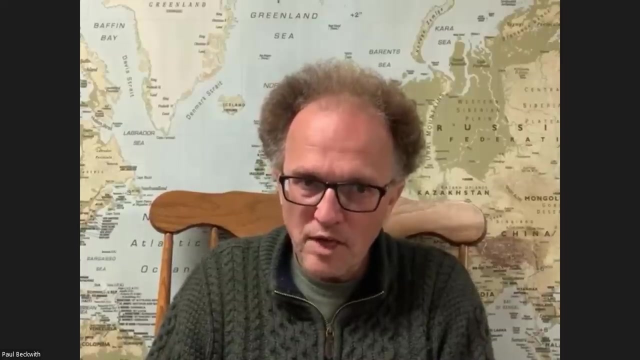 powerful El Nino That also caused the global temperature records. So when we get the next El Nino, on top of the climate change that we've had in the interim since the last strong El Nino, then we're going to blow away records and the chance of exceeding an entire year being above. 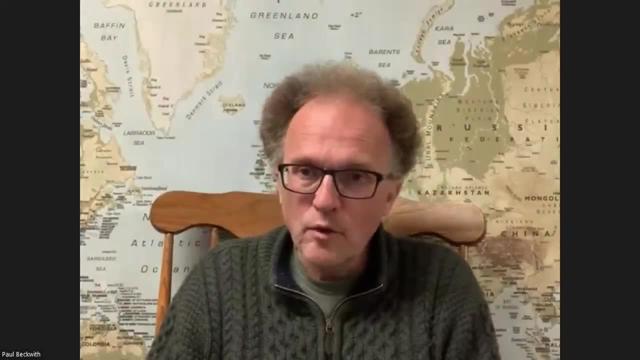 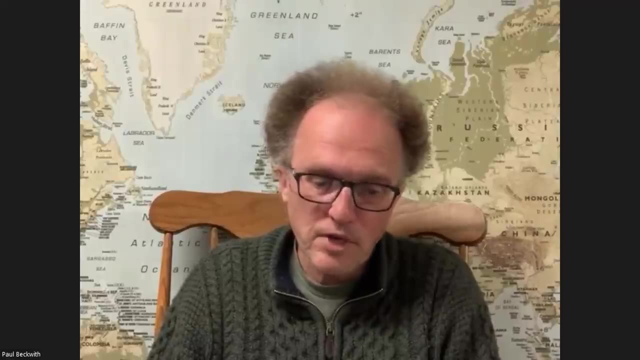 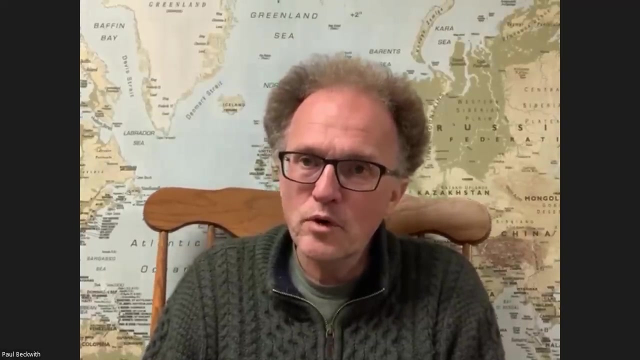 1.5 degrees Celsius is very high. Even back in 2015,- 2016,, we did exceed that 1.5 temperature record in the month of March. Peter said it was 1.66.. The other thing that's important that I should note that people have probably 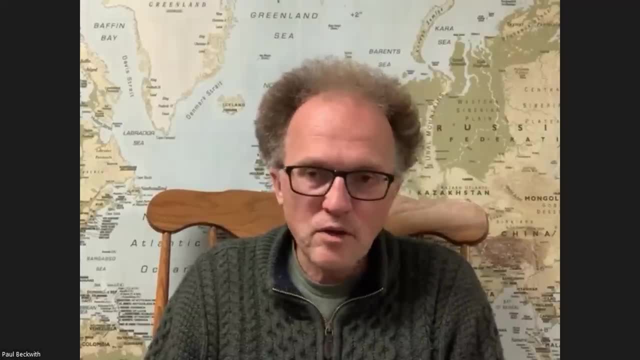 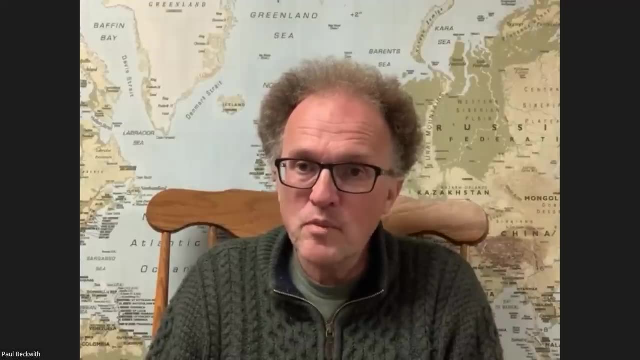 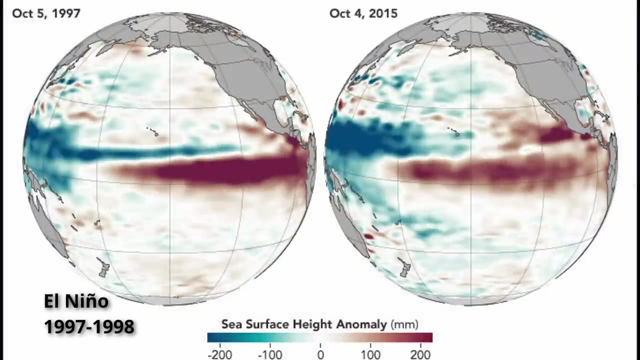 forgotten about is that the deniers used to always say: there's there's been no warming since 1998.. Remember, for the longest time they were pushing that idea- no warming since 1998, and this was pushed for a decade, you know even more, a decade and a half, And then finally, 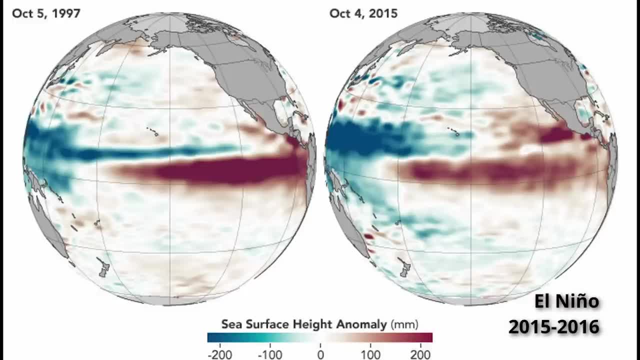 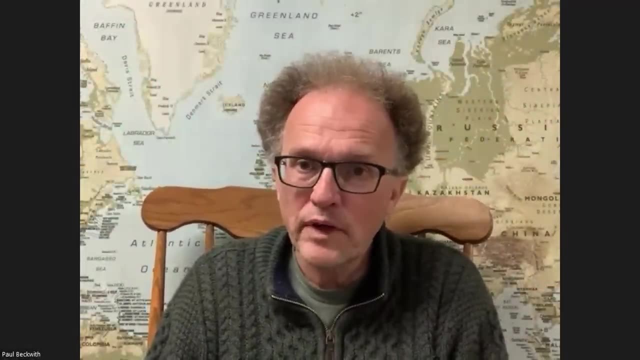 when the 2015, 2016 El Nino came along and blew away the temperature records, that completely quieted and invalidated what the denial people were saying. I don't want to dwell on that, But you know the 1998 was a very powerful El Nino, one of the strongest up until. 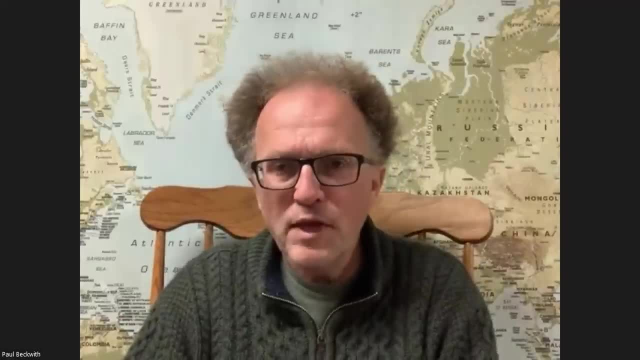 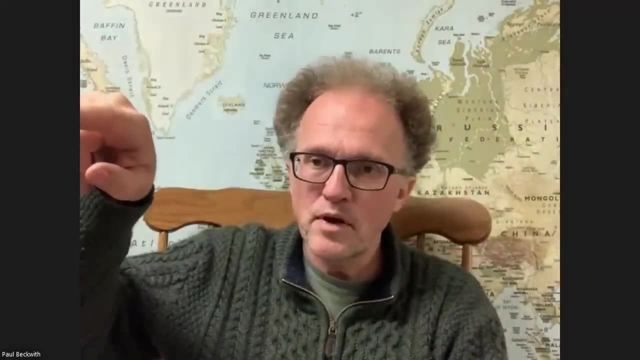 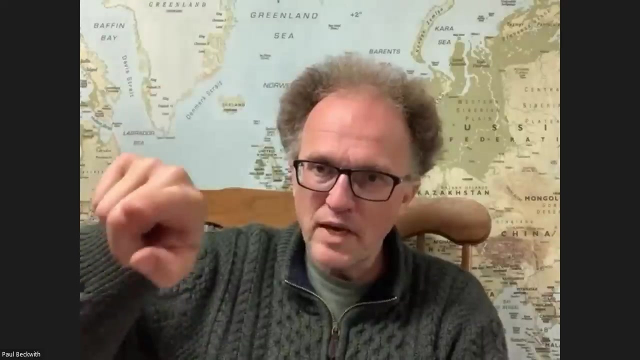 that point. So one of the problems is: think of the climate, think of the temperature rising like this, And then there's fluctuations from year to year depending on whether it's an El Nino or a La Nina year, And when we get the El Nino spike, you know we set all the temperature records and the extreme. 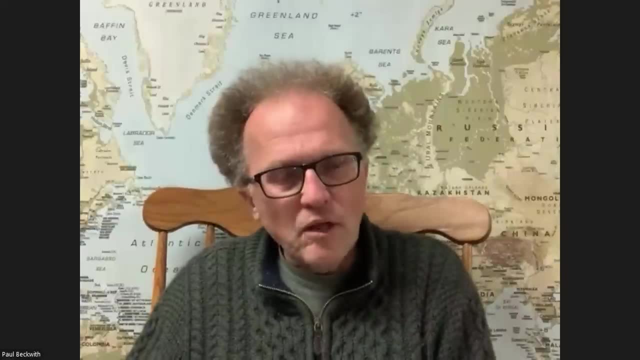 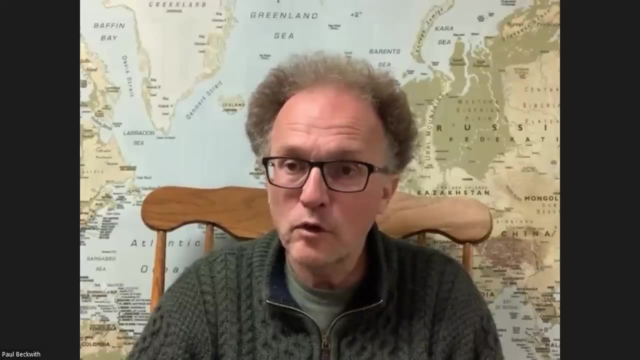 weather events take off around the world. So if we start losing the La Nina state, then the temperature rise around the globe will just be a big problem. So I think that's a big problem And I think we need to accelerate that much more Now. it's not necessarily that that's going to. 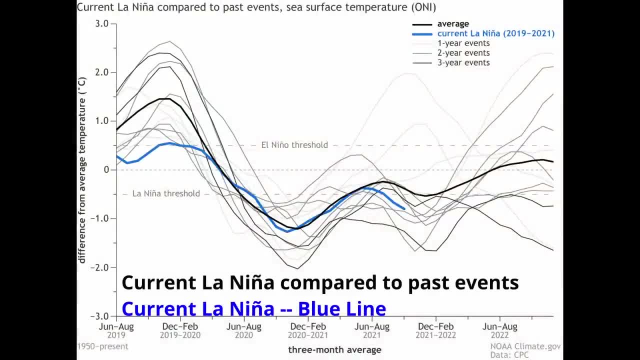 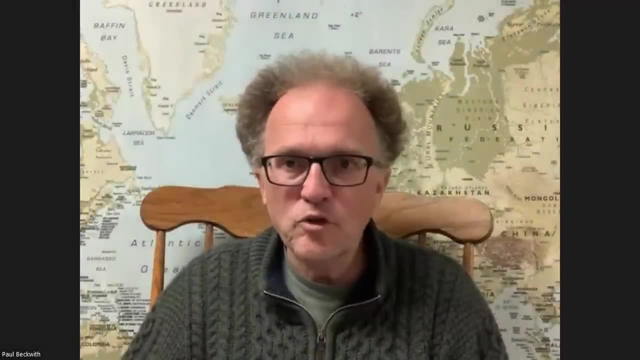 happen. This present La Nina has been very surprising to the people that study this in great depth because it has lasted for, you know, two, almost three years cooling and it's very surprising. You know it's been fairly powerful, But it's very surprising that you know it's. 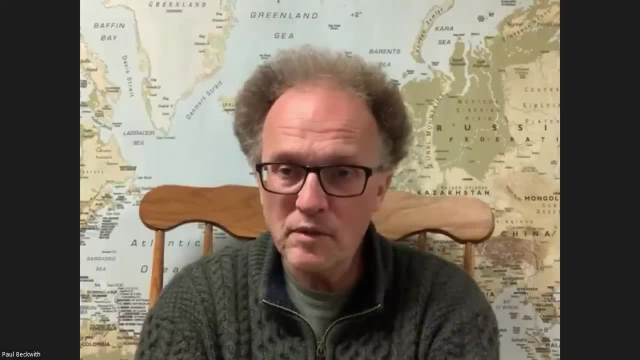 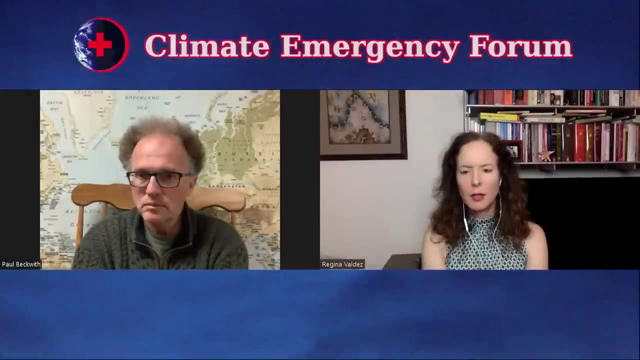 lasted so long, So we need to understand it more, you know, but it's definitely very impactful phenomena in our climate system. Thank you for that, Paul. So, Paul, we've talked about La Nina and El Nino as phenomenon, oscillating trend. Is there something in between? Is there something neutral? I think I heard you. 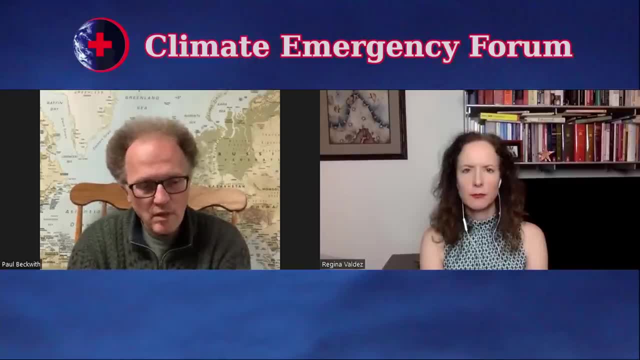 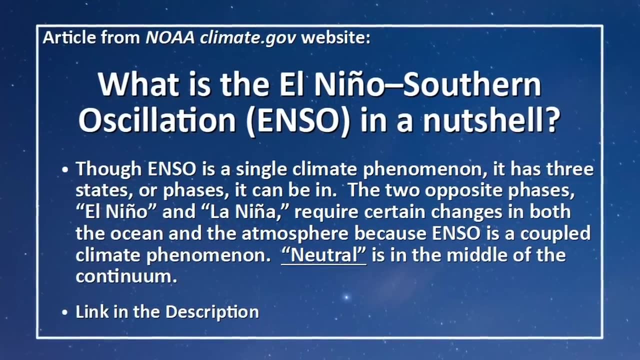 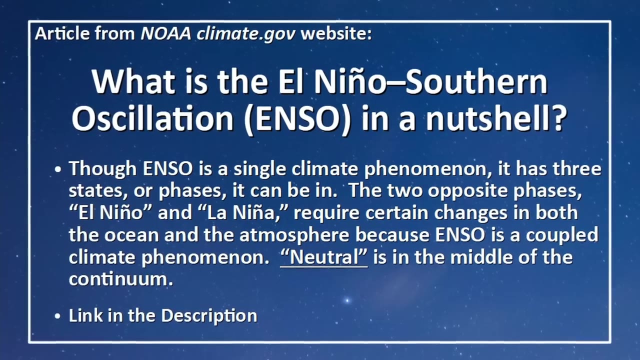 mention that a bit earlier. Yes, So there is a neutral state And sometimes, instead of a full oscillation from an El Nino to a neutral and then to La Nina, sometimes what happens is there's an El Nino and then it goes. 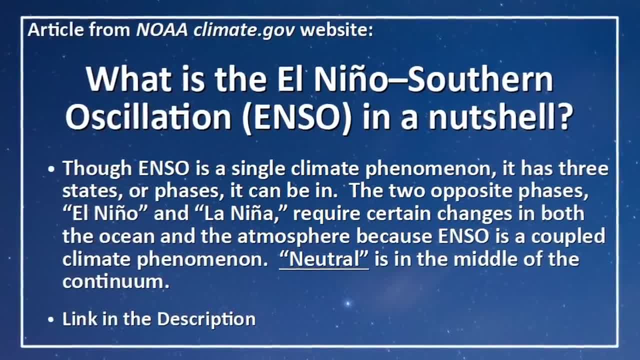 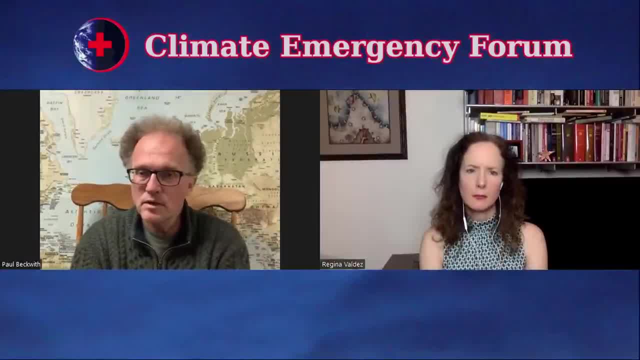 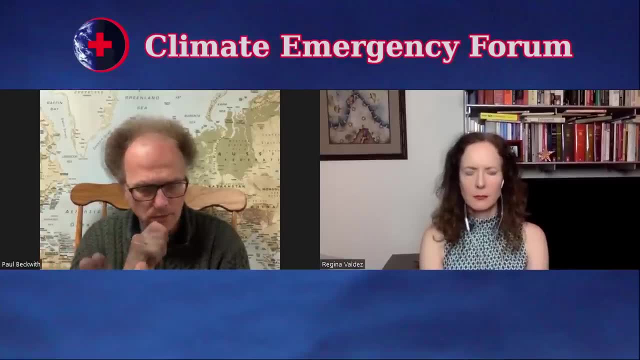 to neutral and then we can get another El Nino without going into the La Nina condition. So that throws another wrench into the whole system. That's why, you know, I don't like to think of it just as a simple oscillation or a pendulum. I describe it more as what a physicist would call a. 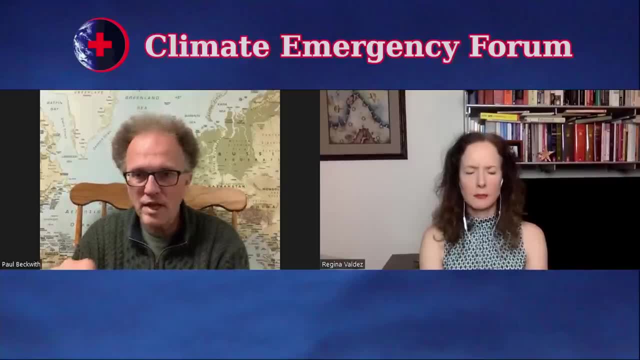 compound pendulum. It's a pendulum where you have other strings attached to the normal what we think is a normal pendulum weight. So it really makes the behavior of the system complex, difficult to model. So the big question is: are these cycles getting more intense with climate change And is the period? 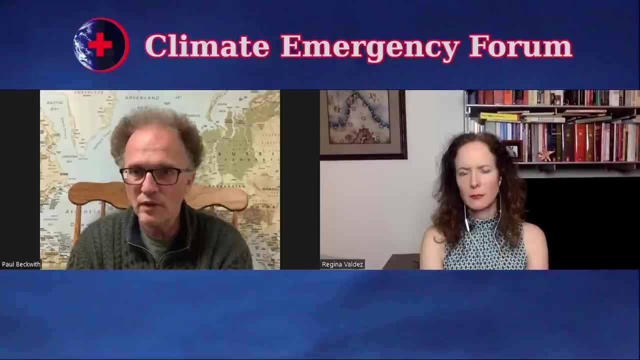 of these cycles changing And are we tending to get more of the El Ninos and less of the La Ninas? And you know, I would say yes to all of those things. Up until a few years ago I would have said that it would be very unexpected to get a strong, long duration La Nina. but we've 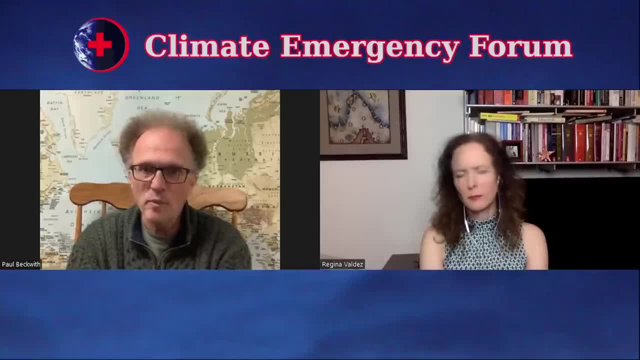 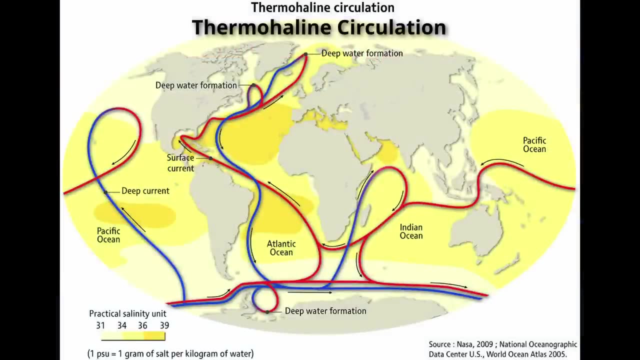 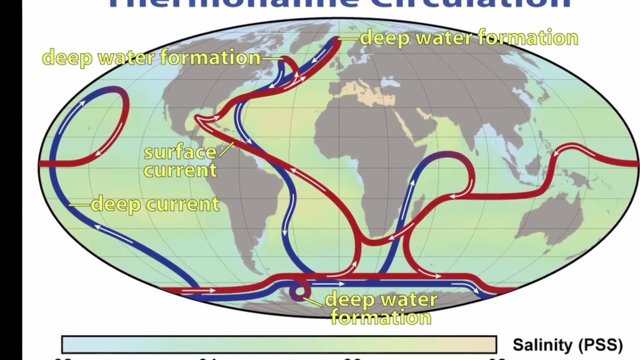 tended. we've had that in the last few years, So we need to think about this a lot more in the context of other ocean things like the thermohaline circulation and the stratification of the water and things like that. It's all tied together as part of the climate system. 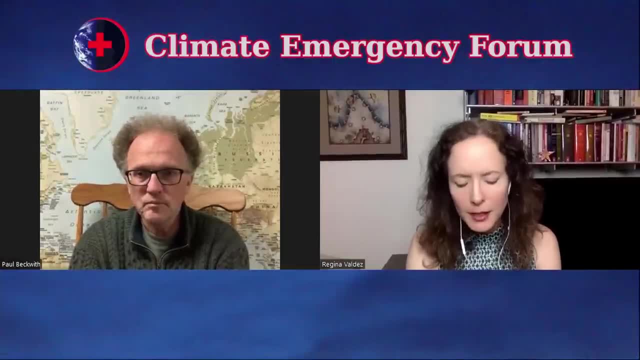 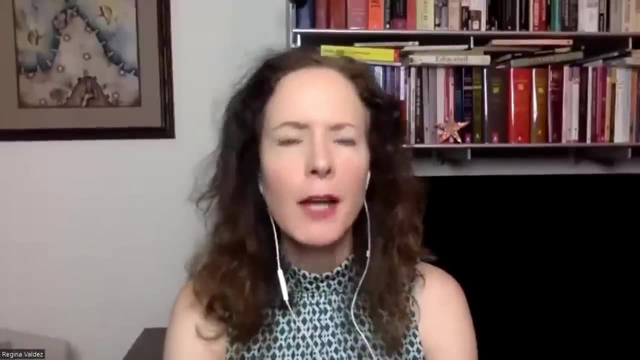 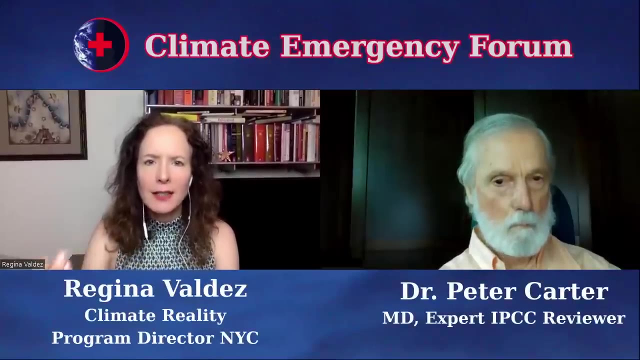 Thank you for clarifying that for us. Paul Peter, you had also mentioned the idea of, you know, increasing El Ninos. I mean, we've got the warming already built in, but then add to that maybe less La Nina. maybe you know some neutral. 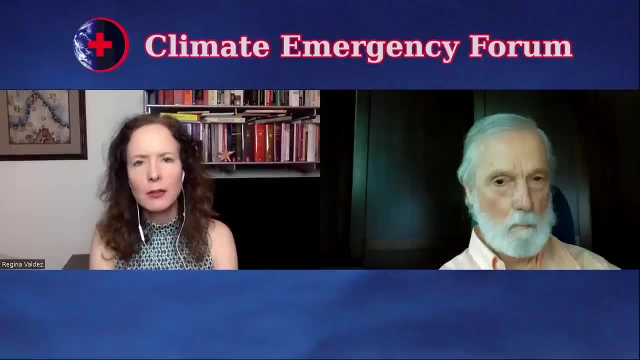 times and greater El Nino, And I think you are on on that path, explaining to us what that could mean for the future. Oh, wait, wait. We all hope that, with these programs that we're doing, we all hope that our governments 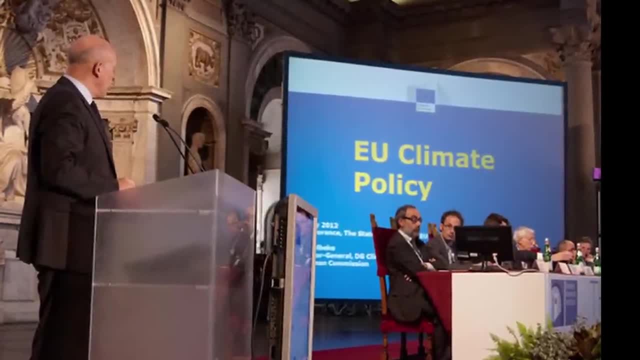 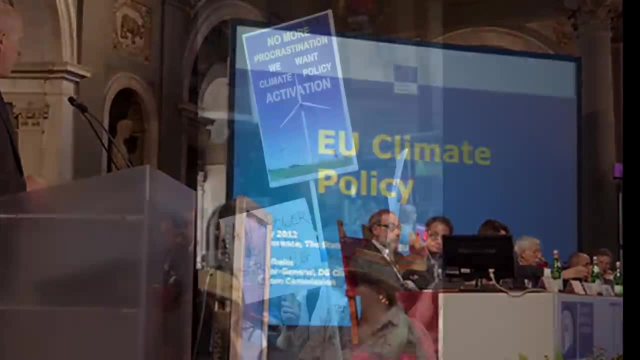 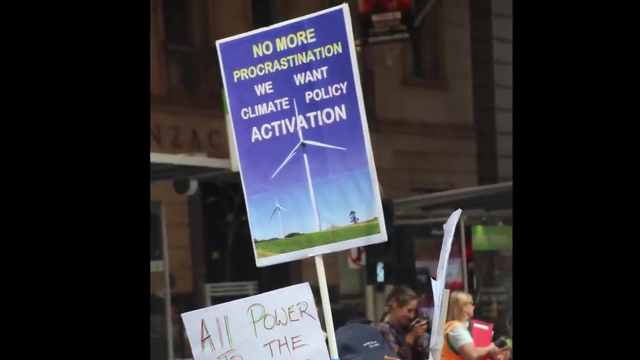 are going to start taking global climate change, global warming, global surface heating and the inevitable- more El Ninos. We are hoping to God that they're going to start taking this seriously because clearly our governments are not doing this at all. So the biggest thing that's driving us: 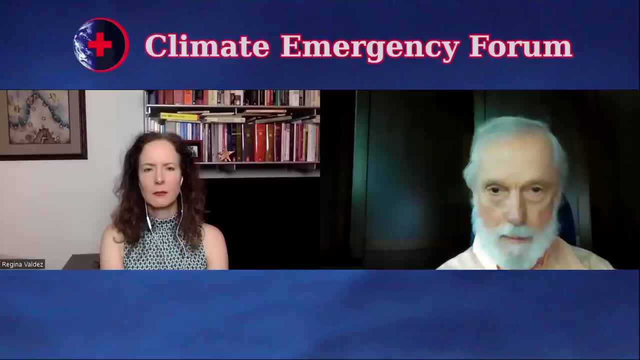 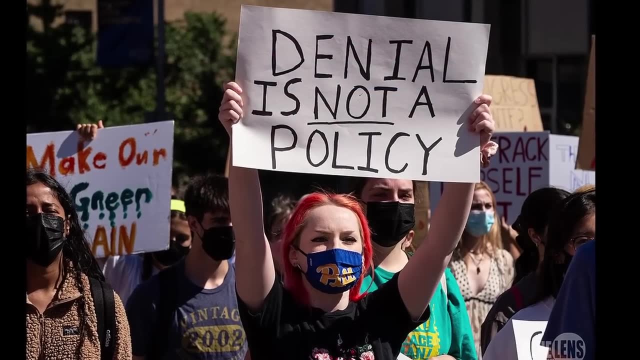 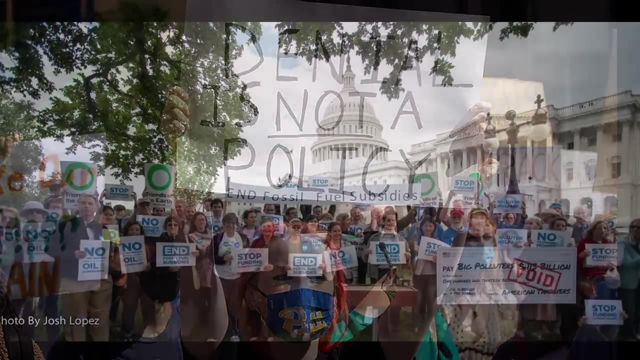 towards catastrophic El Ninos. on top of accelerating global warming is our own governments. So that is the worst, strongest driver towards climate catastrophe. because they're not taking this seriously at all, They're continuing to subsidize fossil fuels, Even the European Union. 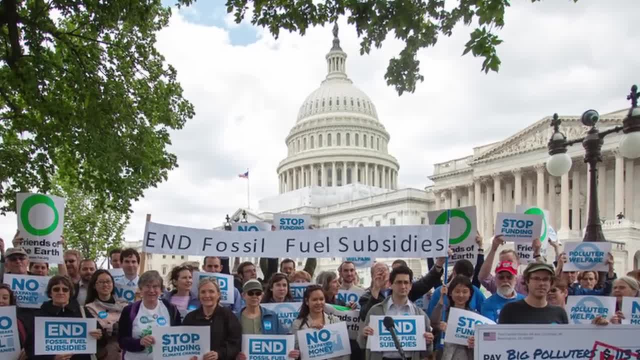 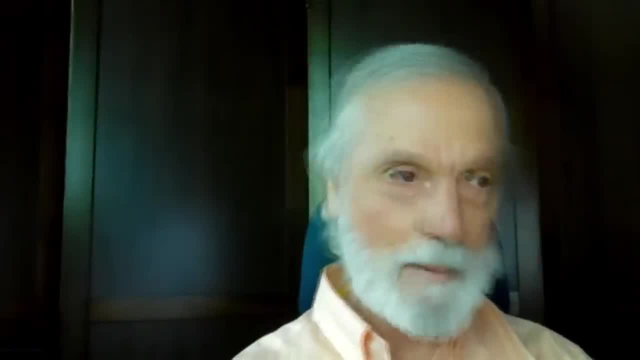 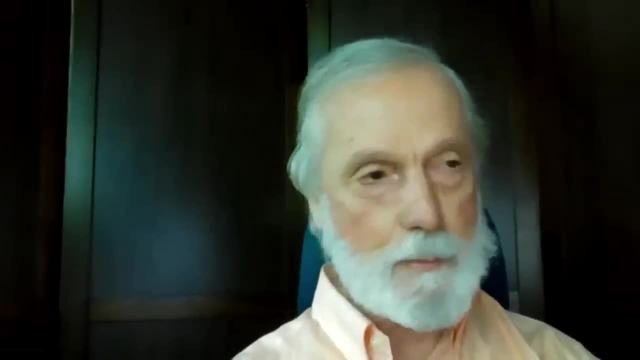 their fossil fuel use and their emissions have already increased above the pre-COVID 2019.. So that would be my, my wish. I want to mention again, though, what we, what we will expect with the El Nino In the 2015-16,. there were three massive forest fires burning across the globe. 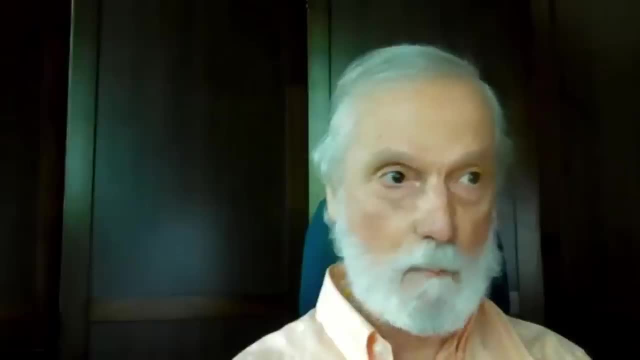 The Amazon was. the Amazon fired up a lot more. The forests of Central Africa were also burning, And in Indonesia, those fires which are which we're used to, they flamed up a lot, A lot higher. Now, right now, land carbon sink is beginning to, at least beginning to switch. 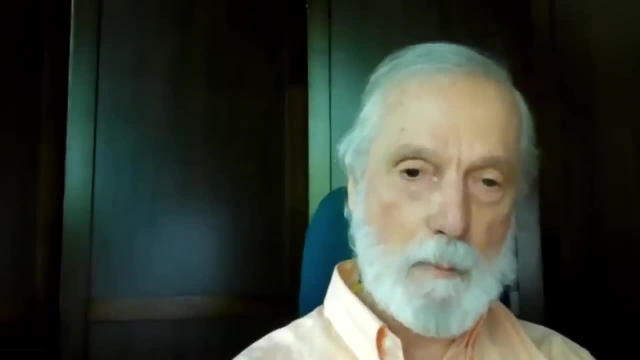 With the next El Nino, we're going to have the forests being a huge source of more CO2, not a sink. They're going to be a huge source. So we're going to see this big jump in atmospheric CO2, much greater than the last El Nino, And so the global temperature. 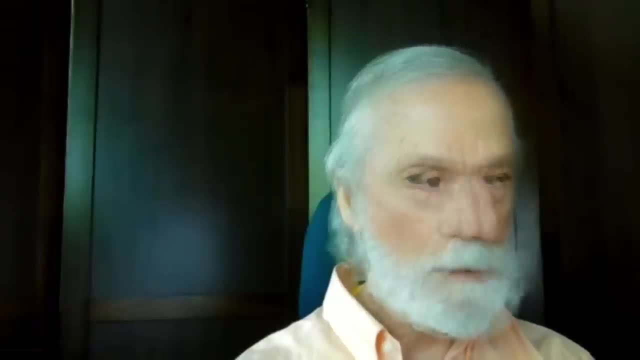 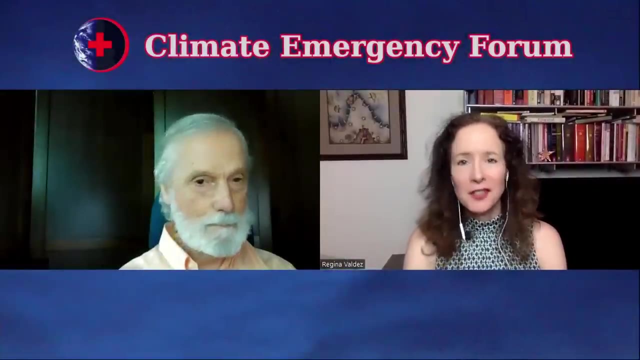 increase will almost certainly be even more. We've got to get this across to those damn governments of ours. Thank you, We're running out of time. So what does it take? You know, one wonders what does it take. It seems like people don't move and tell forests to move. 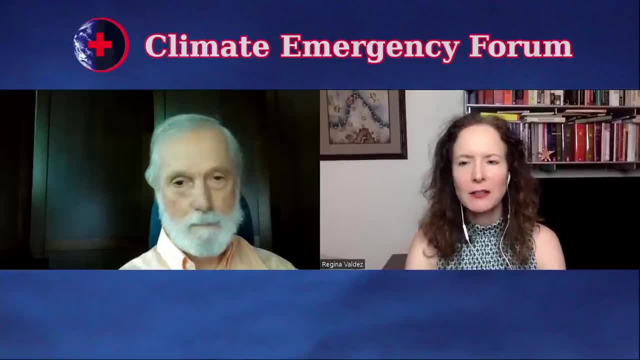 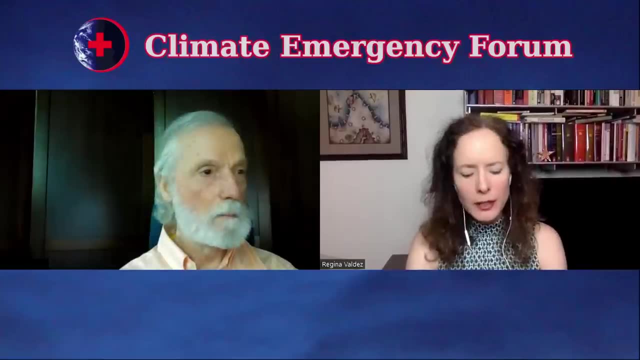 but the difficult thing is, in this situation, if we decide to move when we're forced to move, well, by then it may be too late. So before we we close, I'm just wondering if you have anything else to add, Paul, on this topic. I know it's one that's near and dear to your heart. 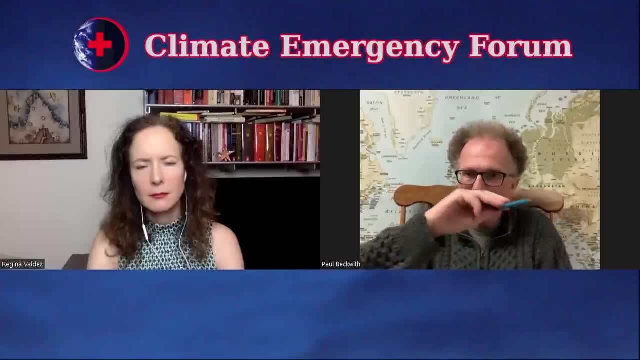 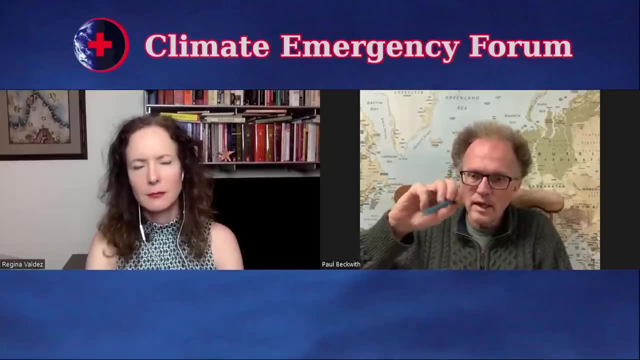 Yes, So I mentioned that, the. you know, we have a temperature rise from climate change and then we have the fluctuation on top of it from the La Nina, El Nino, And there's a lot of questions as to whether the El Nino fluctuations will end up going higher and last longer, or 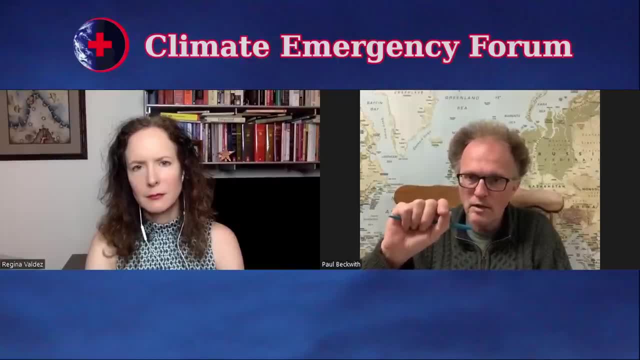 you know, occur more often as opposed to the La Ninas, But one thing to remember is that the climate system is is tightly coupled. There's lots of different systems that are that are reliant on other systems And the risk is that you know a very powerful El Nino, long duration El Nino. 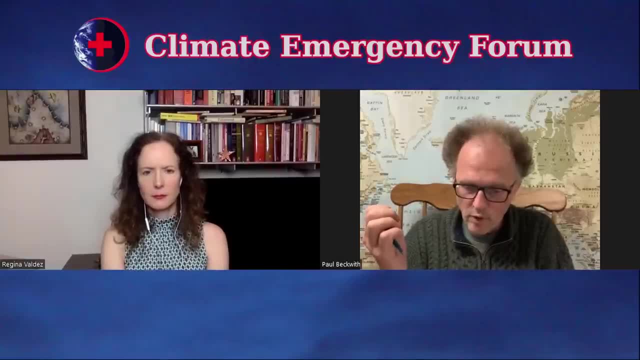 breaks other parts of the climate system, for example, causes tremendous fires in the Amazon, completely destroying its ability to absorb carbon when the El Nino passes right. So then we would have some irreversible- at least on short human time scales- breakage of the system. Or if you think of the oceans, you know the next. 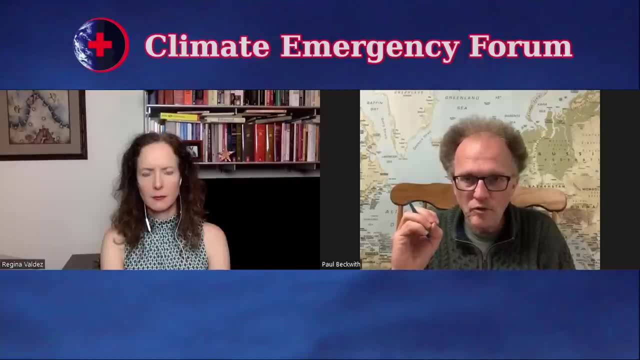 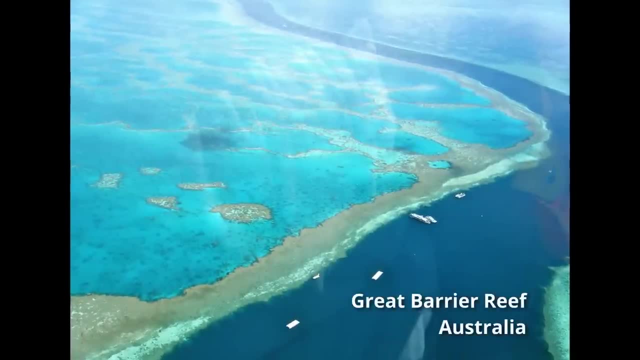 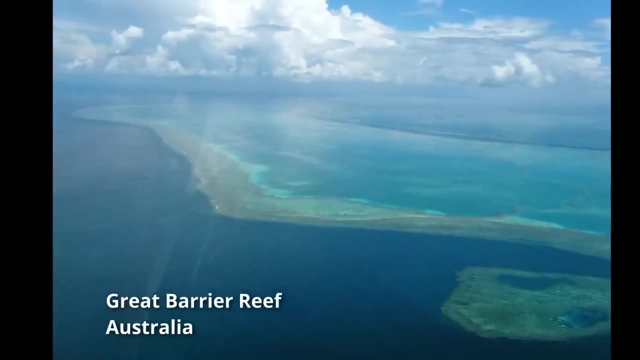 very powerful El Nino can cause enough sea surface temperature warming, say in Australia, to completely finish off the Great Barrier Reef. And then, when the El Nino year passes, there's no Barrier Reef left right. So you know these sort of fluctuations on top of the ongoing rapid climate change are very, very concerning and very, very, very significant to a lot of the anti-climatic industries in Australia and we've found that ''DISCLAIMER'', I think, the issue of the big breakage of the system or, if you think, of the oceans, 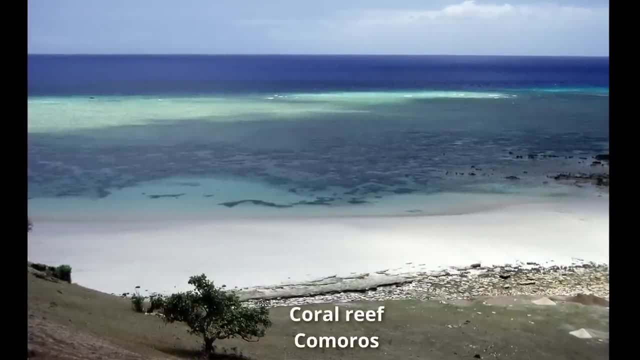 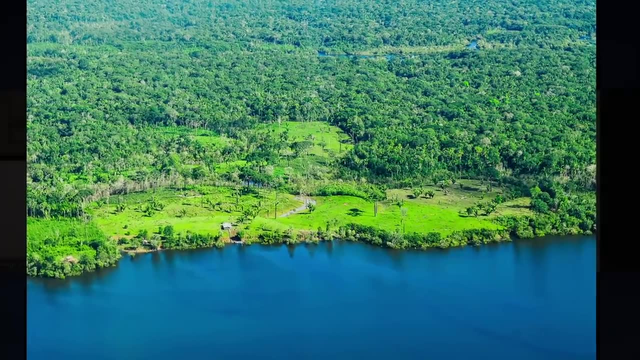 you know, the next very powerful El Nino can cause enough sea surface temperature warming, say in Australia, are very, very concerning and very, very risky for damaging huge systems that are necessary, like the coral reefs or the Amazon rainforest. Yes, you bring up very grave repercussions from 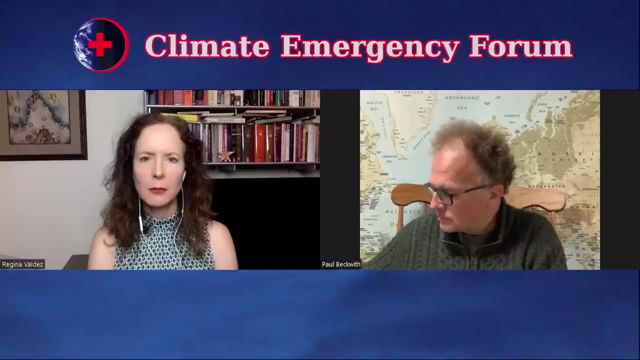 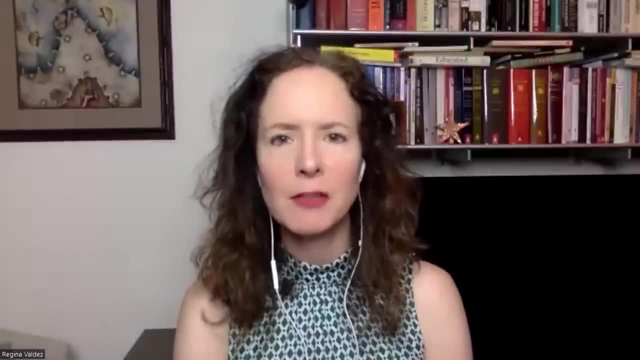 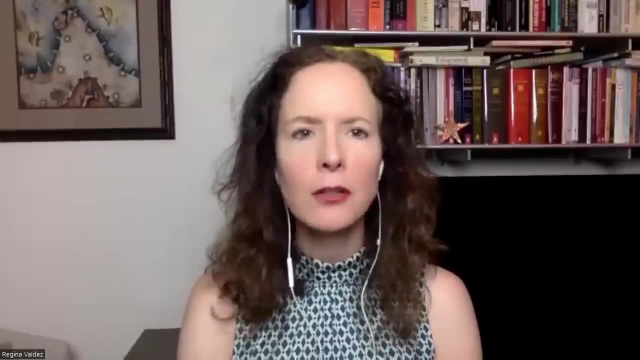 this, And I think it's fair to say that we're all witness to something very historical on our planet, something that our species hasn't seen before, but definitely something that we've had a lot to do with. Thank you for bringing up feedbacks And thank you, all of you, for staying.